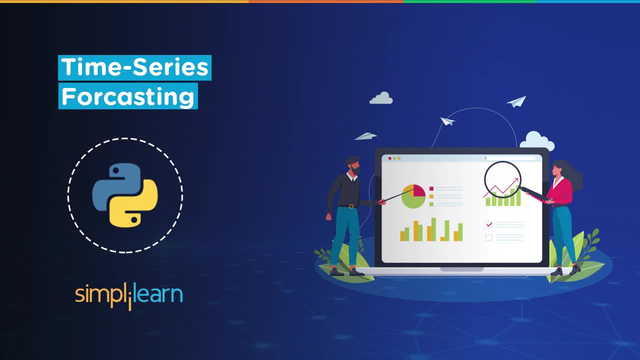 type in: yes. If there are any issues, do let us know in the chat section so that we can resolve them. Let's wait for some more minutes to let other people join. Let me tell you, guys, that we have regular updates on multiple technologies, If you are. 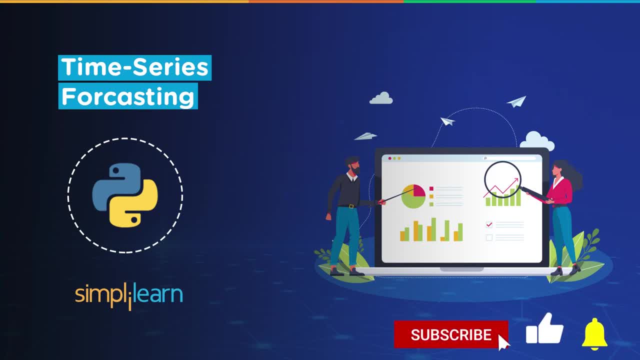 a tech geek in a continuous hunt for the latest technological trends, then subscribe to our YouTube channel and press that bell icon to never miss any update from Simply Learn Great. I think we can get started. So in today's session we will discuss what time. 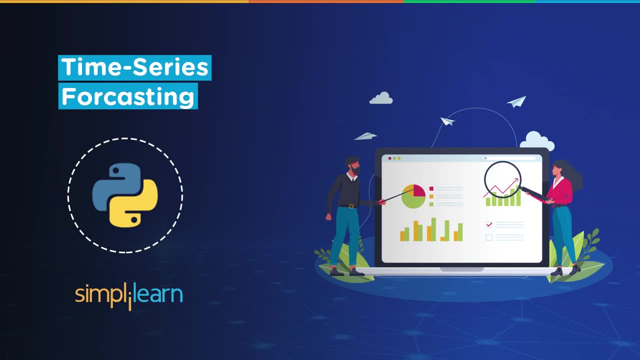 series forecasting is After that a hands-off lab demo of how you can do time series forecasting using machine learning. We will perform different functions and different Python libraries for analyzing the data. Before we move on to the programming parts, let's discuss time. 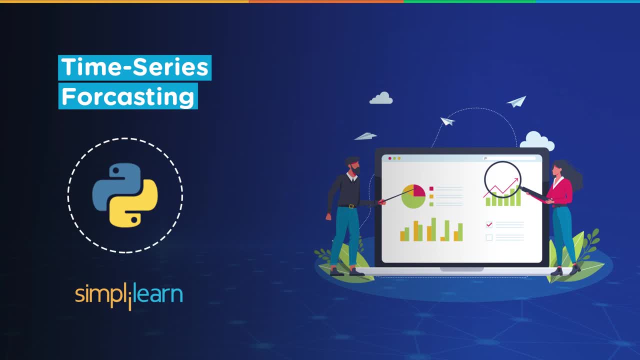 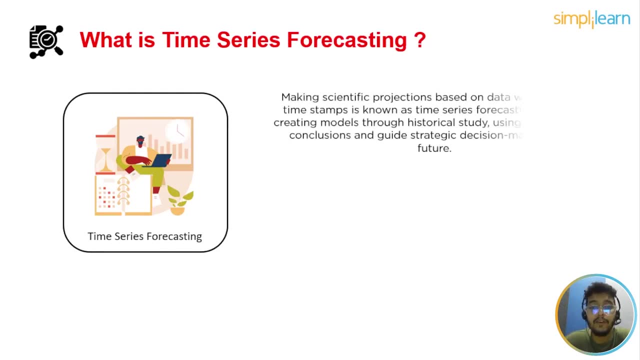 series forecasting and proceed further for the same. What is Time Series Forecasting? Making scientific projection based on the data, with historical timestamps, is known as time series forecasting. It entails creating models through historical study, using them to draw conclusions based on time series forecasting. This is what time. 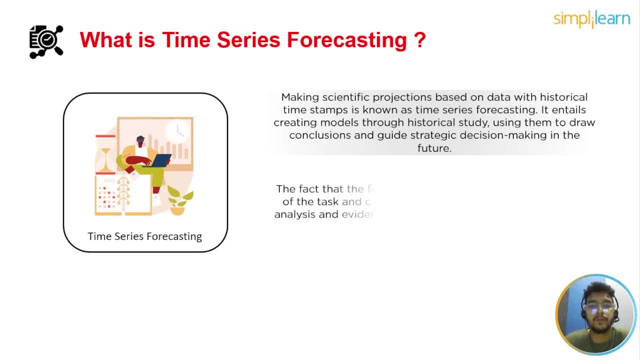 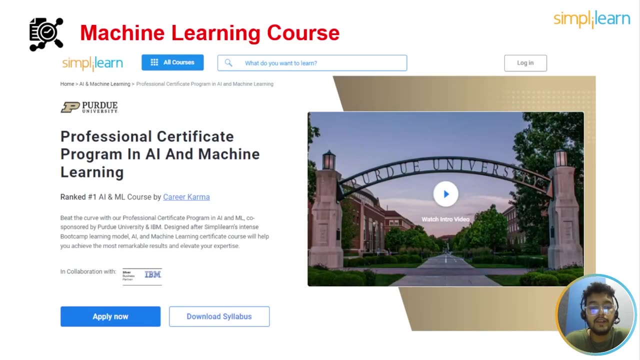 conclusion and guide strategic decision-making in the future. The fact that the future result is wholly unknown at the time of the task and can only be anticipated through analysis and evidence-based priors is an essential distinction in forecasting. Give yourself a chance to simply learn. Professional Certificate program in AI and Machine Learning. 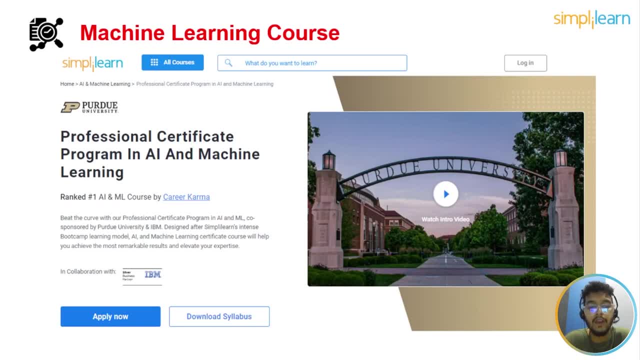 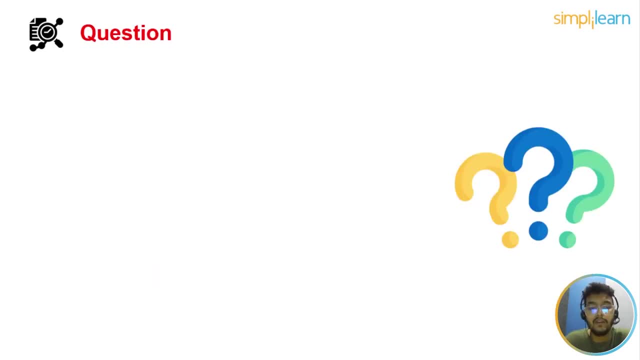 which comes with Completion Certificate and in-depth knowledge of AI and Machine Learning. Check this course details from the description box below. So here is one question for you guys. I will give you exactly one minute for this. You can comment or you can give your answer in the chat section. 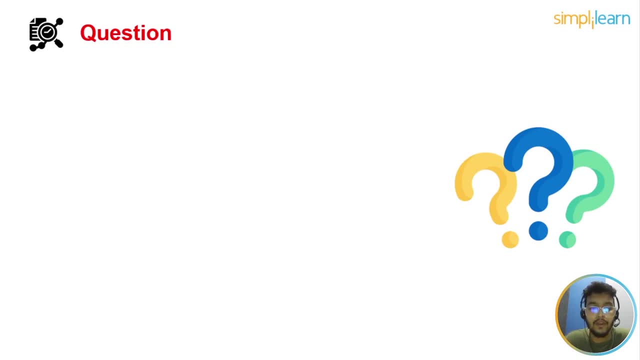 So I can see if the answers given by you are right or wrong. So the question is: which type of programming does python support? I am repeating again: which type of programming does python support? Option A: Object-oriented programming. Option B: Structured programming. Option C: 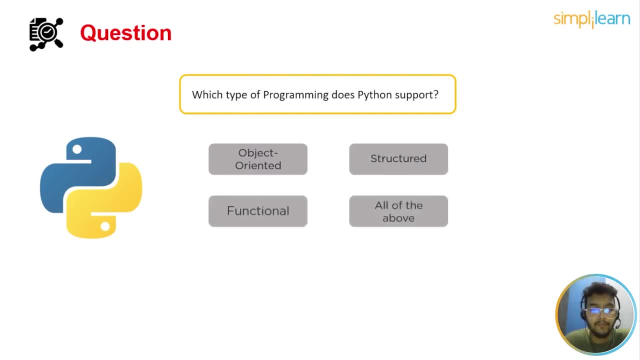 Option D: Functional programming, Option D- All of the above. So let us know your answer in the chat section or in the comment section. So I am starting a timer of one minute. just type your answer in the comment section or in the chat section. 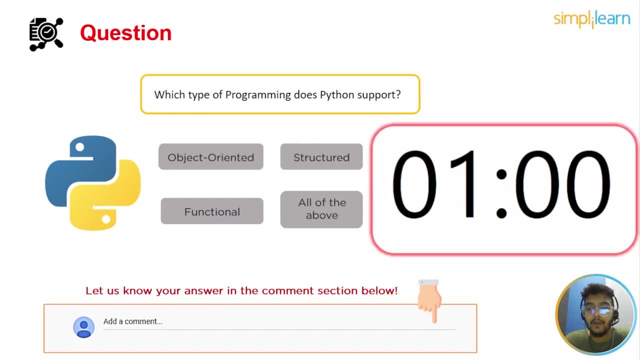 Do let me know your answers, please. So I am starting the timer of one minute. Which type of programming does python support? Object-oriented, Structured programming, Functional or All of the above? You can comment or you can give your answer in the chat section. 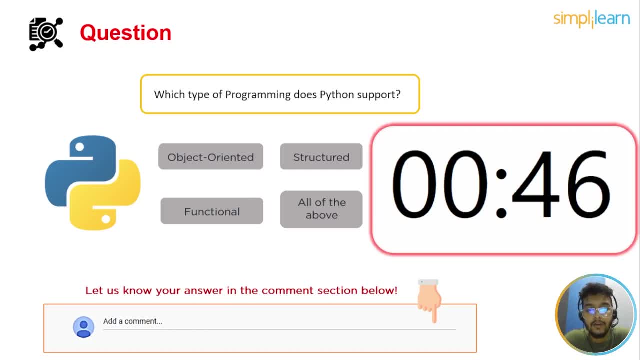 So I can see if the answers given by you are right or wrong. Which type of programming does python support? Object-oriented, Structured, Functional or All of the above? Thirty seconds meaning: Which type of programming does python support Object-oriented? Which type of programming does Python support Object-oriented? Structured, Functional or all of the above? 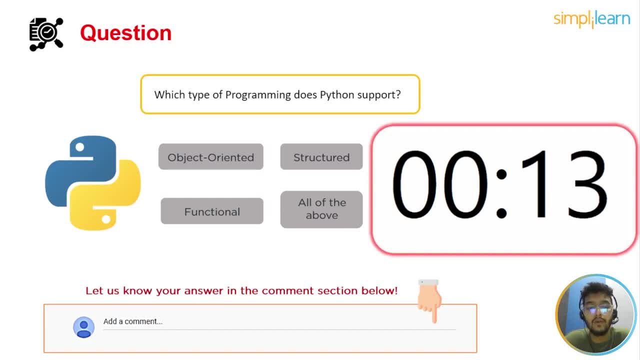 Let us know your answers in the chat section or in the comment section below 10 seconds more. Which type of programming does Python support 5 seconds more? So the allotted time is over. We will give a reply to those who gave the correct answer. 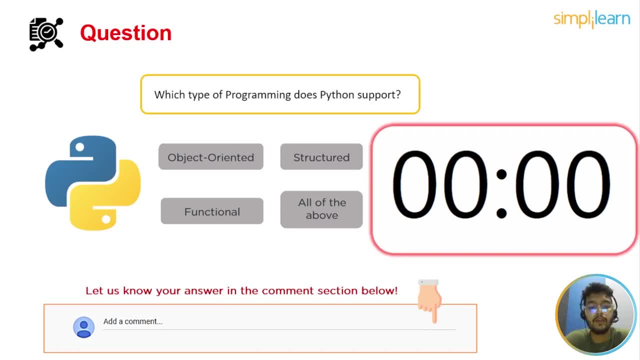 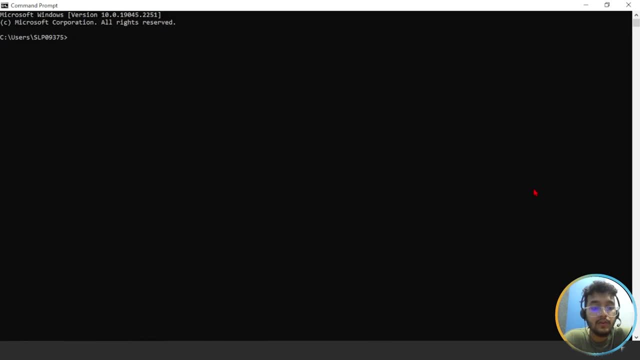 and for those who didn't give the correct answer, We will give you reply with the correct answer. Okay, Now let's move to our programming part. So we will open command prompt to write a command to open Jupyter notebook. So here I will write. 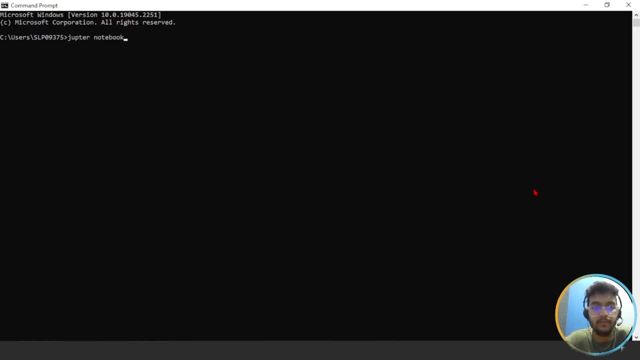 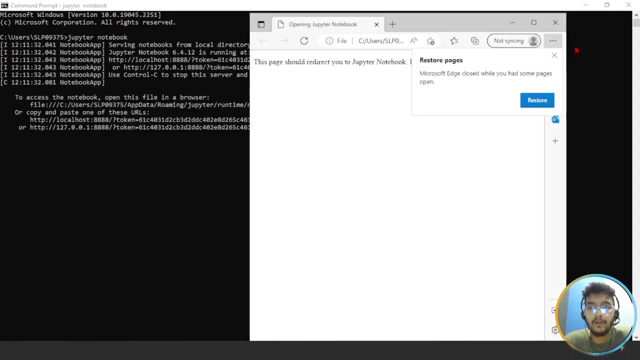 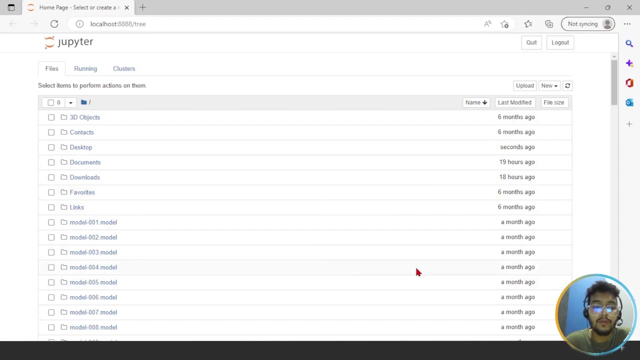 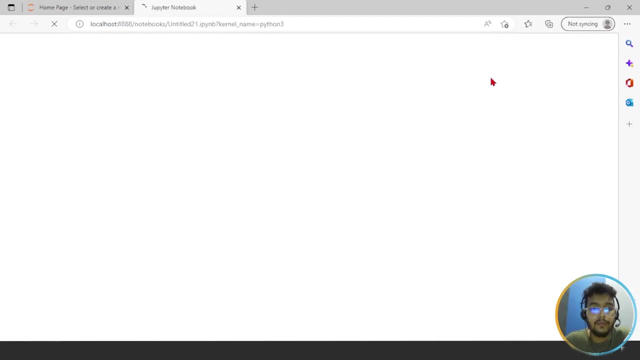 Jupyter Notebook Press. Ok, Jupyter Notebook- press enter. It will take time. It's open. So this is the landing page of Jupyter Notebook, and here I will select new Python kernel file. So this is how Jupyter kernel look likes. 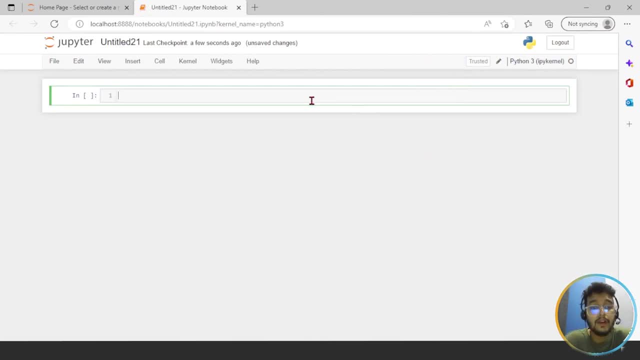 So here what we will do: we will import some major libraries of Python which will help us in analyzing the data. Okay, import numpy as NP. Okay, then import pandas as PD, Then import Seaborn as SNS. Both one is from. 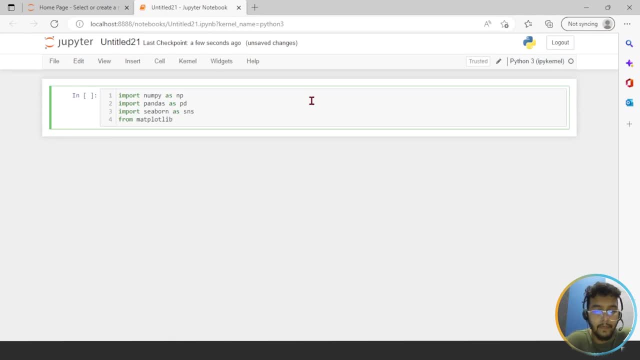 matplotlib, Both pyplot as PLT. Okay, then we will import some model libraries. So here I will add: from stats models or TSA dot API Import exponential smoothing and comma than simple XP smoothing. Then one more: Hold, We will write here: import. 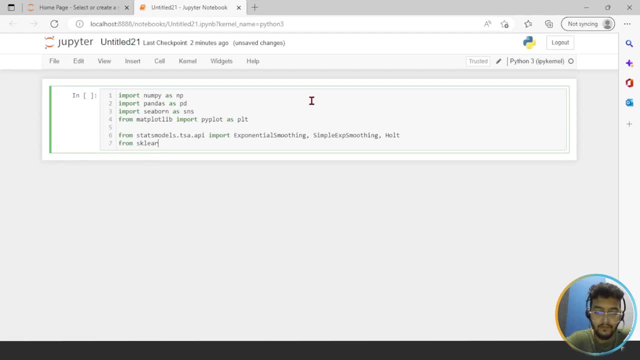 Sorry from SK. learn dot: linear Underscore model. Import Linear Gretchen. Okay then import warnings. Then we will write here: warnings, dot filter warnings. It should be ignore. Yes, there will be no error, We're still loading. 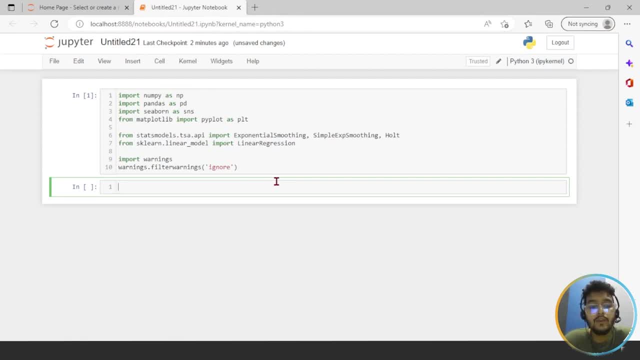 Yeah, So numpy. numpy is a python library used for working with arrays. It also has a function for working with the domain of Lineal Algebra and matrices. It is an open source project and you can use it freely. numpy stand for numerical python. Second is Panda. 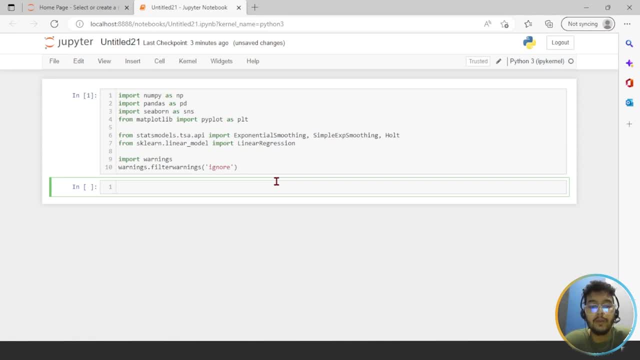 Pandas is a software library written for the python programming language for data manipulation and analysis. in particular, It offers data structure and operations for manipulating numerical data and time series. Then seaborn, an open source python library based on matplotlib, is called seaborn. It is utilized for data exploration and data visualization. 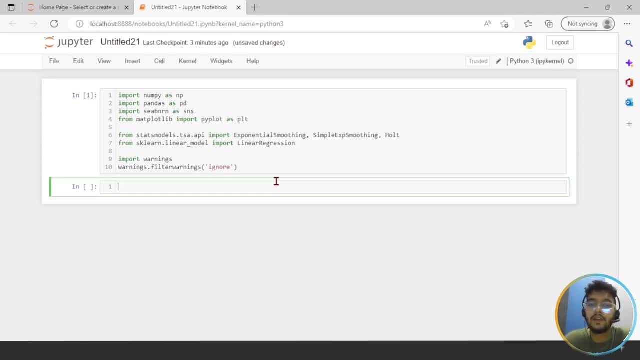 With data frames and the pandas library, seaborn function with ease. matplotlib for python and its numerical extension, numpy matplotlib is a cross-platform data visualization And graphical charting package. as a result, it presents a strong open source substitute for matplotlib. The APIs for matplotlib allow programmers to incorporate graphs into GUI applications. 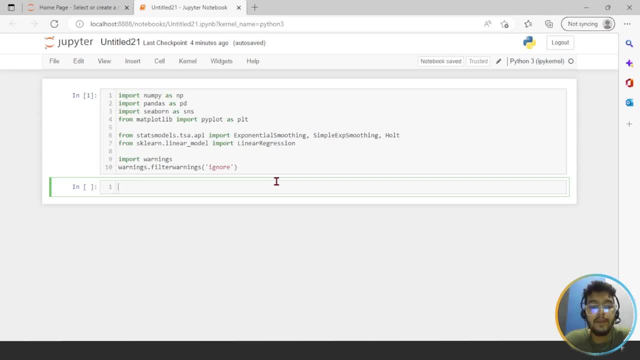 Linear regression- the machine learning method regression built on linear supervised learning Analysis, regression is done. Regression creates a value for the aim prediction using independent variables as inputs. It main goal is to investigate the relationship between factors and forecasting. Exponential smoothing: The exponential windows function is a general method for smoothing time series data, known as exponential smoothing. 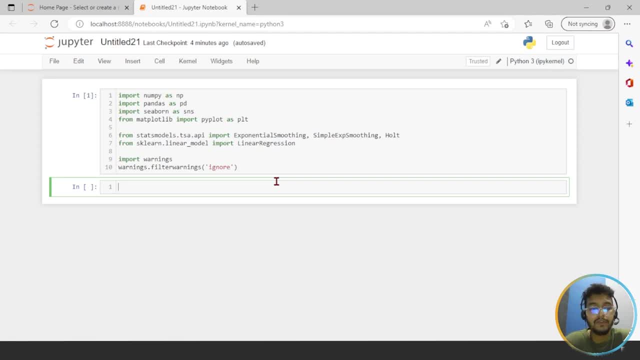 It contrasts to the ordinary moving average, which weights previous data quality. Exponential function: use weights that decrease exponentially with time. And there is one more simple, exponential smoothing. The simple exponential smoothing classes use simple exponential smoothing models to give very simple time series analysis. 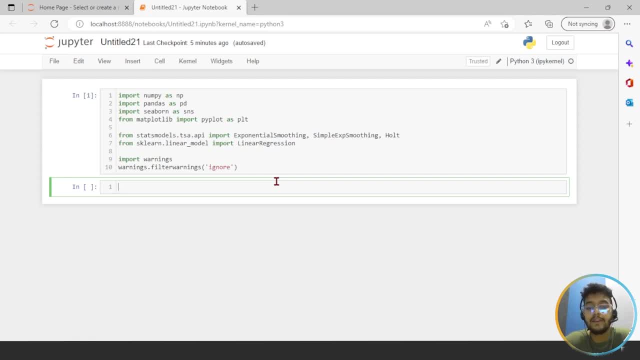 A weight average of the most recent value and the preceding smooth value constitute the predicted value. The contribution of older value degrade exponentially as a result of the smoothing parameter. Okay, so after importing libraries, let's import data set. For this I will write here: dfr. 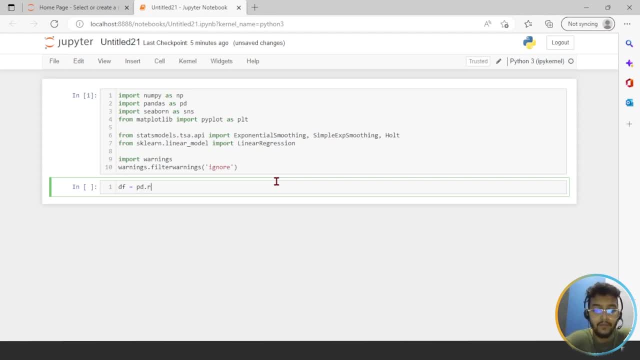 name: pdedcsv. here I will write monthly underscore: csv dot csv. Okay, this is my file name. You can download this file from the description box below And for seeing the data I will write here: df head. Then press enter. 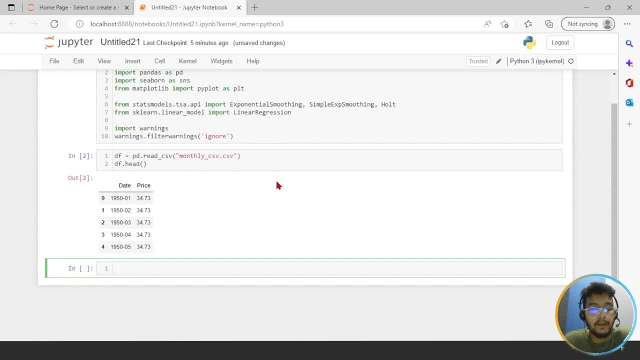 Yeah, So here, pd is for pandas library, Read is used for reading the data set from the machine and csv is used for the type of file which you are using, Okay, or which you want to read. And if you want to see the top five rows of your data set, you can use head. 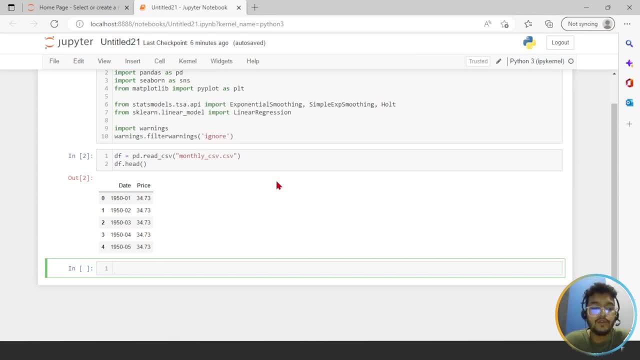 And if you want to see the last five rows of your data set, you can use tail instead of head. Okay, this one, you can write here tail. So moving forward, let's see how many rows and columns are present in our data set. 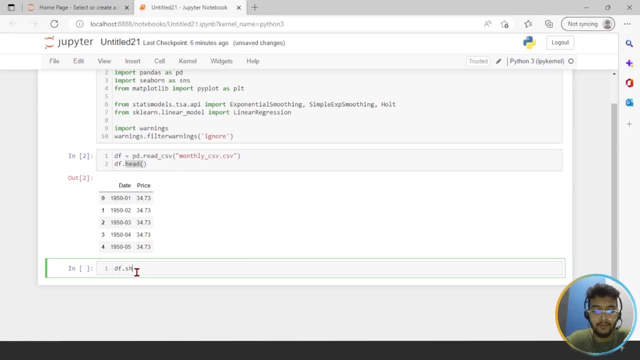 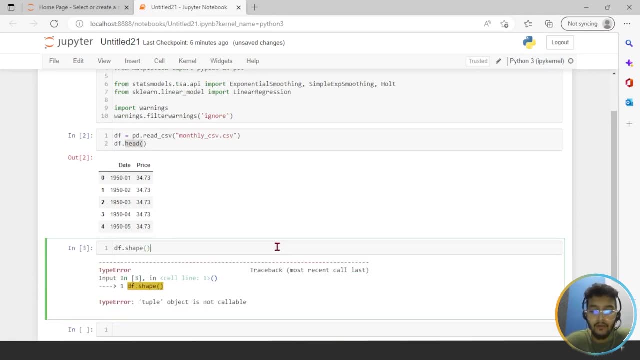 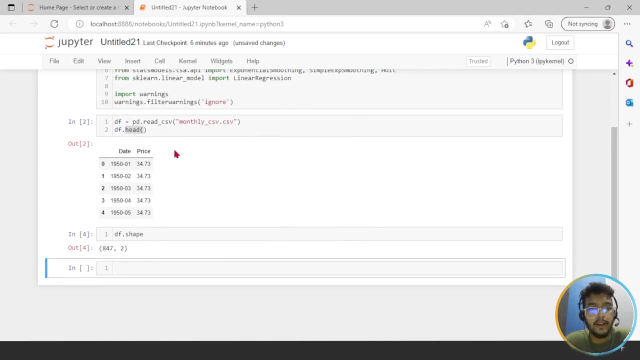 For that I have to write df dot shape, Okay, Then press enter. Okay, it will give error. Why? Because this, Yeah. So here you can see 847 rows and two columns: date and price only. So, moving forward, let's do some EDA: exploratory data analysis. 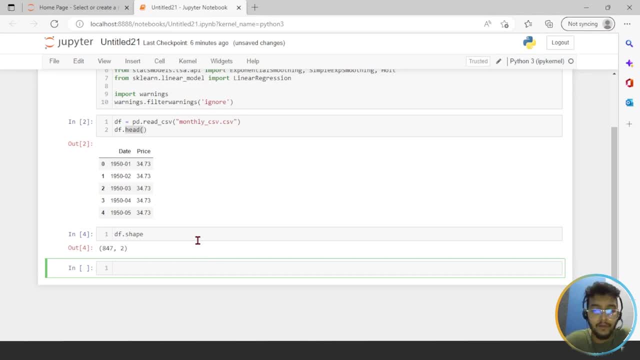 Okay, For that I have to write here print Data Date range Of Of gold prices Available from, And here I have to give curly brackets And df dot location, LOC And colon Comma Date. Okay. 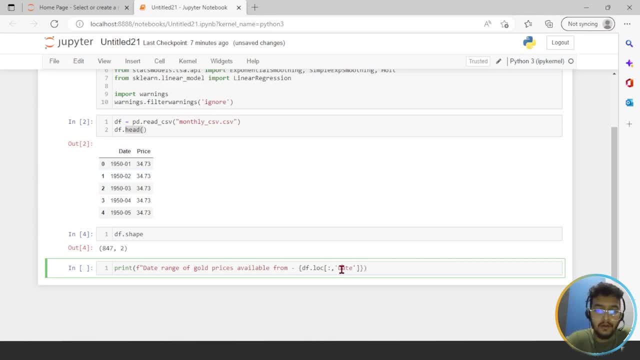 D is capital here, So I have to write Date From location zero. Two, Again same thing: df dot LOC. Date to the length of EF minus one. Oh, everything seems good. Yeah, Then press enter. Okay. 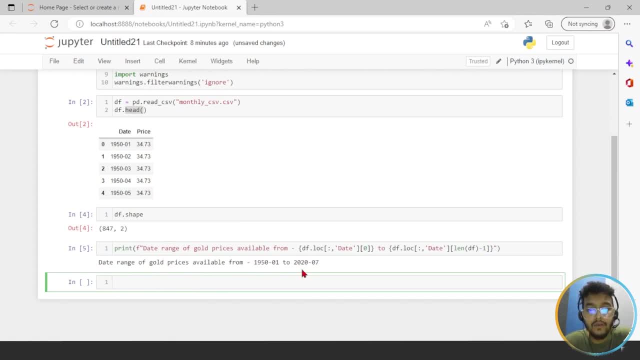 We have date range of gold prices available from this 1950 to 2020.. Okay, in our data set, And here I will write, date equals to PD dot date range. Start from slash one, slash 1950 comma and it goes to eight slash one, slash 2020. 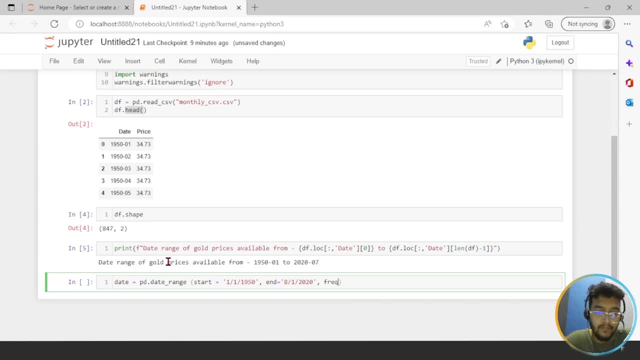 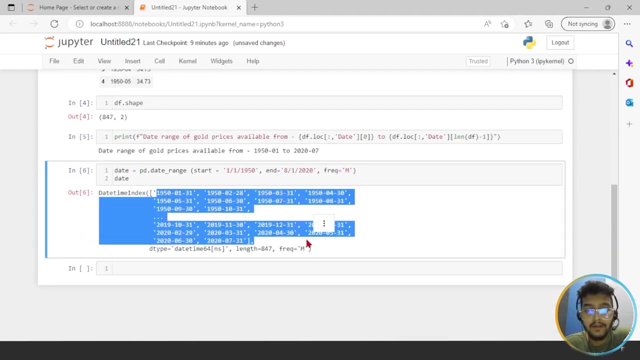 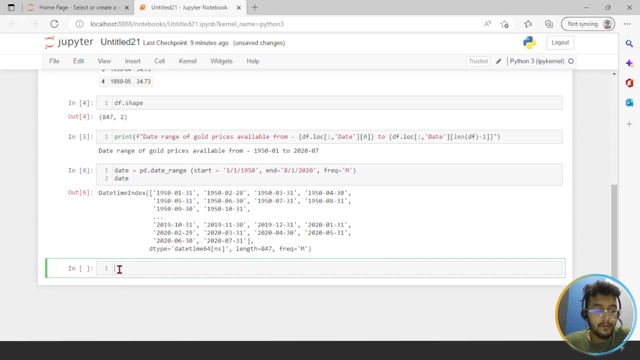 comma frequency was medium, Then then here I will write date and press enter yeah, so here you can see it, date time index. okay, from starting to land these daughters, and here I will write DF and was to date you have taught: drop state comma axis is one. 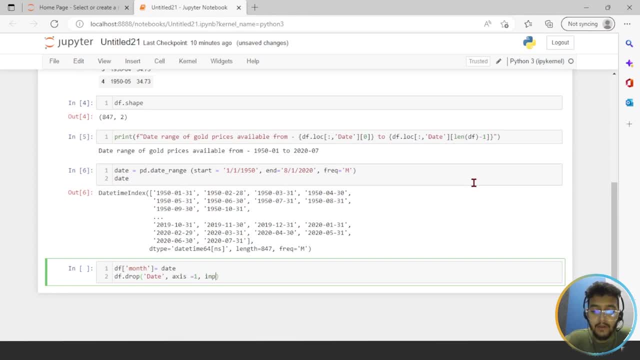 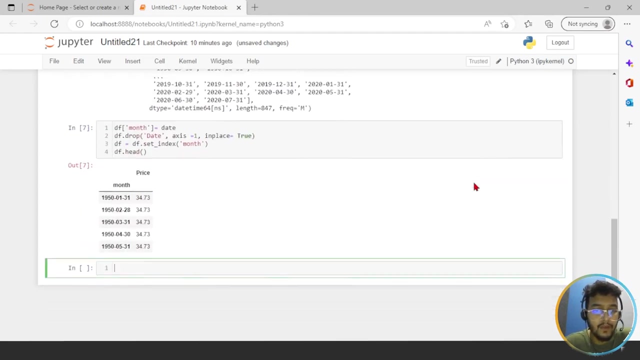 comma in place was true, he should be capital. then DF equals to DF dot set index and month and DF dot head. let's enter instead of this date: you have a desert this month. ok, for particular value, though moving forward, let's see the graph. different, different graphs. okay, 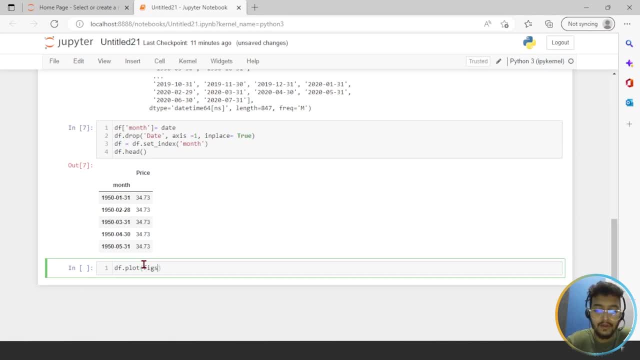 you have to plot and figures are set. should be was to 20 comma it and plot dot title is like gold prices Italy since 1950 and onwards. get that. it should be this. then X level should be plt- dot. x Label, be months, then PLT- dot y levels. 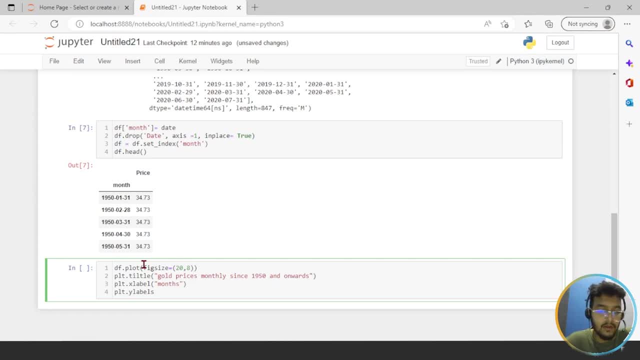 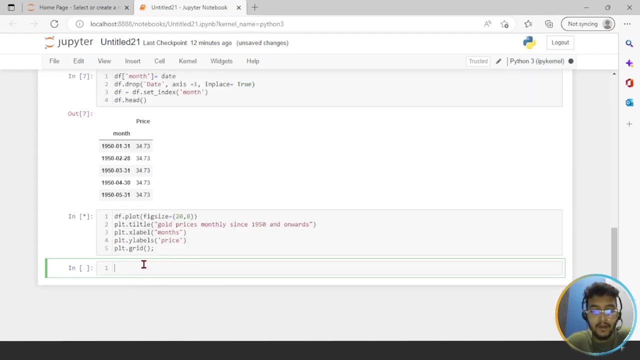 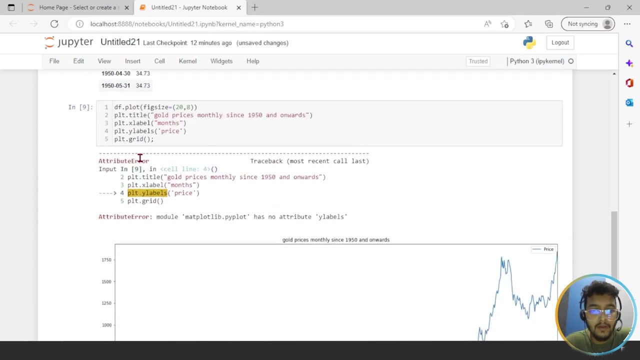 will be months. then difference will be: now, dot, dot, dot. y levels will be'll be x, las come should be price and i will write here: plt dot grid. okay, press enter. okay, title spelling: my bad t-i-t-l-e. okay. then press enter: oh y label. it is sorry. 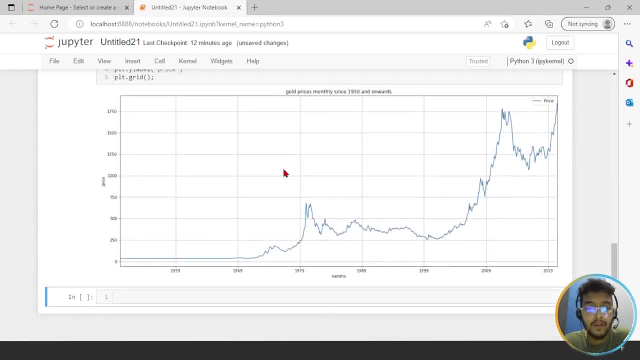 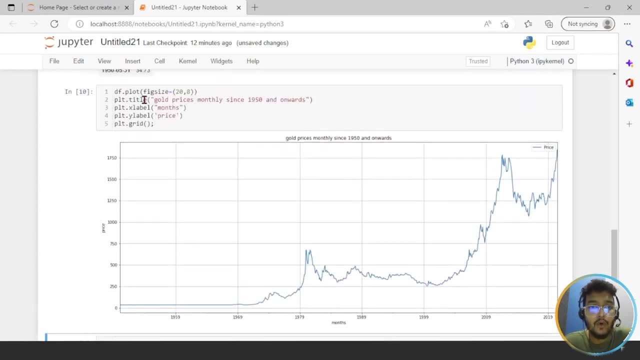 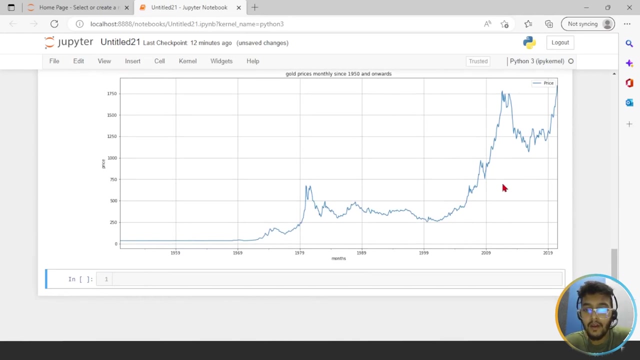 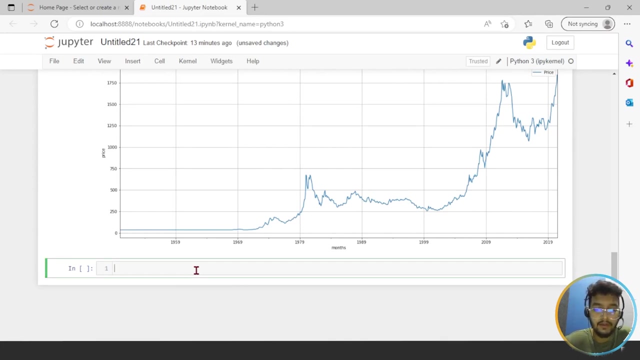 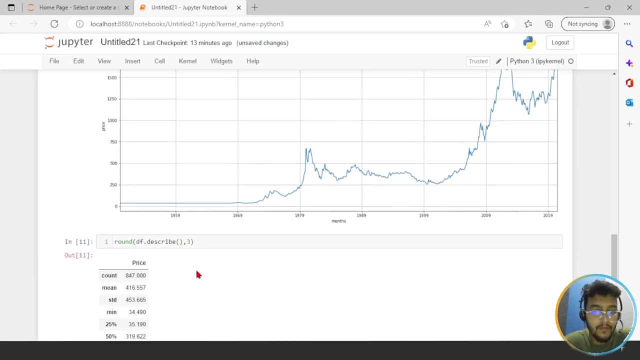 yeah, here you can see gold prices monthly since 1950 and onwards, okay, till from 1950 and from till 2020. okay, this is the price. then, moving forward, let's see another graph. so i will write here for that round df dot. describe comma three. 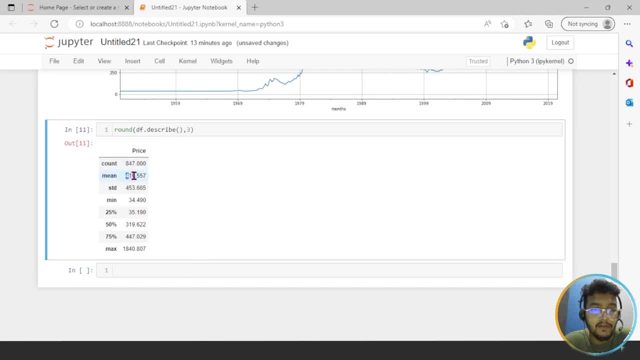 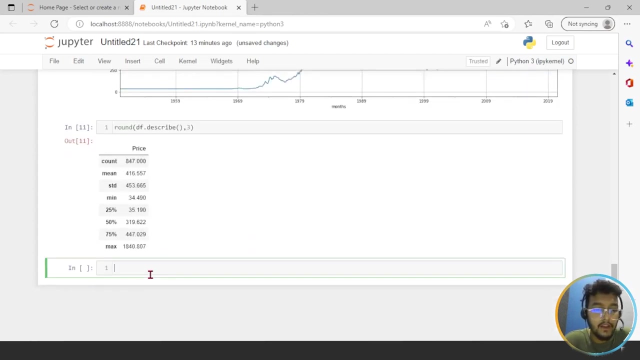 and here you can see the count variable and the average is 416.557. standard deviation. that minimum price value is this: 20 percent this and the maximum value is this: okay. so so the average gold price in last 70 years is this: 416.557, okay. 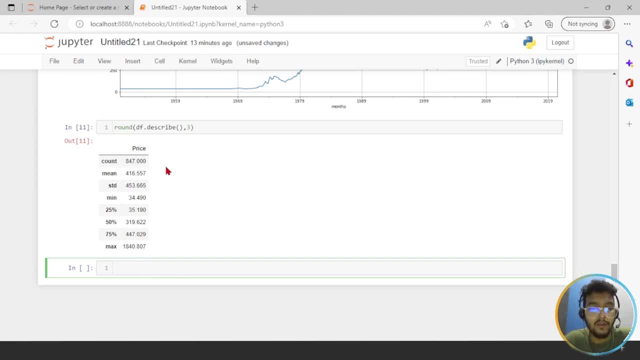 only 25 percent of the time the gold price is above 447. the highest gold price ever touched is this one: 1840 807. so we will do visual analysis. so here i will write: ax equals to plt, dot subplots, subplots. okay, then the figure size. 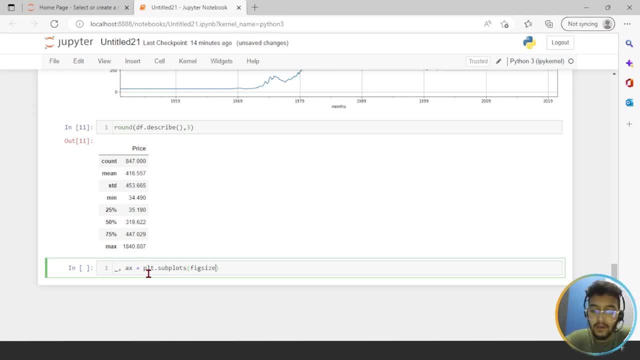 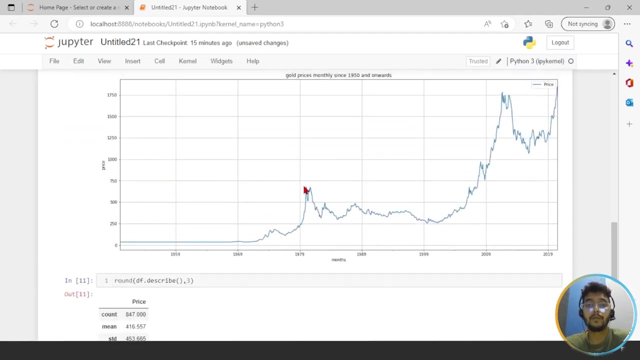 was to 25 comma art. okay, then sns dot box plot is x equals to df dot index dot here, comma y equals to df dot values, okay, 0. my ax equals to x. okay, sum x value안. Then same PLT dot title, gold price monthly 1950, same graph will come, but in the different. 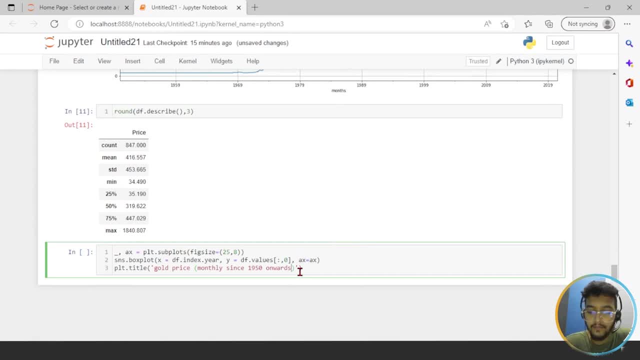 format. okay, Let me remove this. Then PLT dot x label label must be here, PLT dot y label- ice and PLT dot x text will be rotation. okay, I will give rotation 90, PLT dot grid. 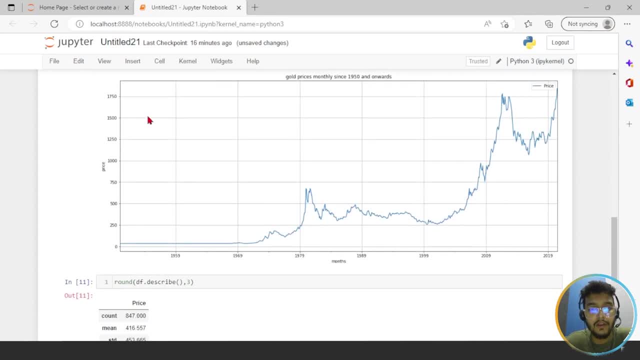 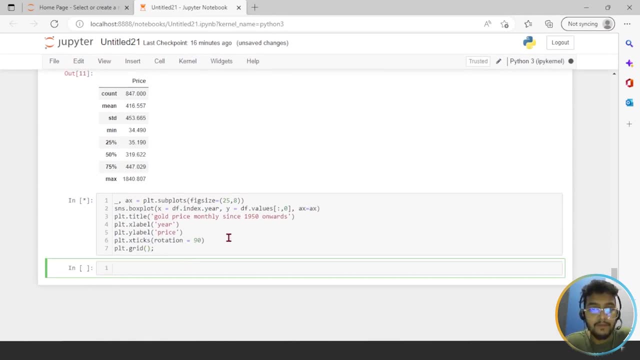 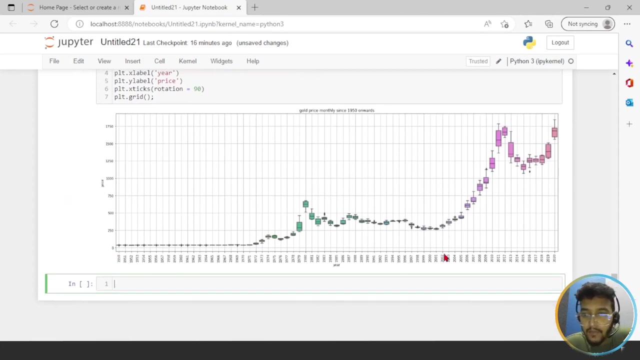 Can write here instead of grid. I can write here directly: show. So grid is With this format, this box format, okay, So press enter. It's loading, Yeah, So here you can see from 1950, every year is here till 2020.. 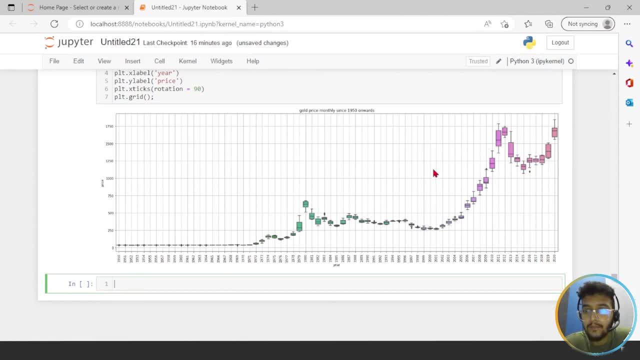 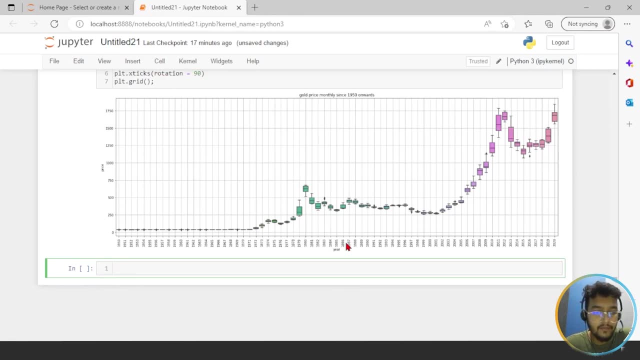 So how the gold prices are decreasing and increasing. okay, Let's see the another graph. I will write here. I will write here from that's: models, models, dot graphics, dot TSA plots, quote, month plot. Okay, Then I will write here: figure AX equals to and PLT dot subplots: bigger size equals. 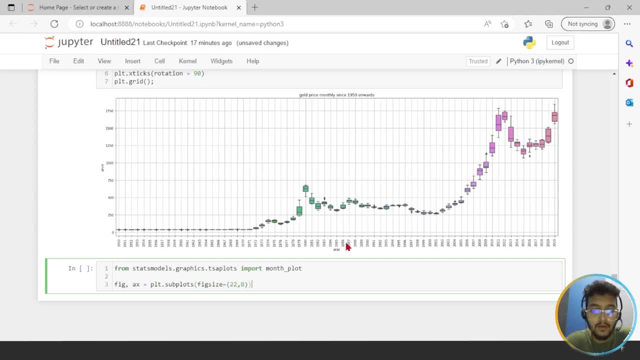 to 22,, eight, Okay, Then month plot: Yes, Y label, Okay. So gold price, okay, comma. then X equals to X and I will give the title PLT dot title. So I will copy from here. No, I'll copy from Phoenix. 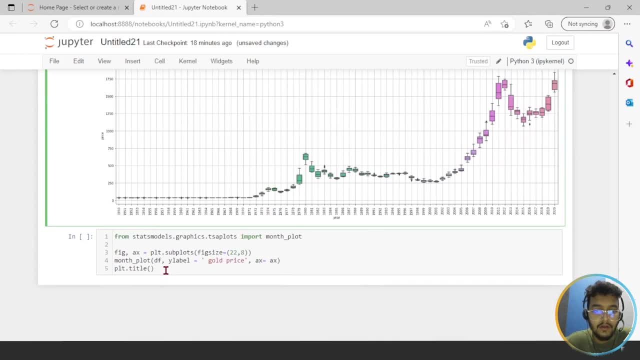 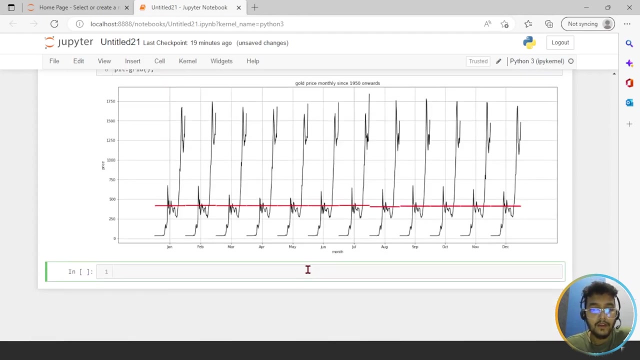 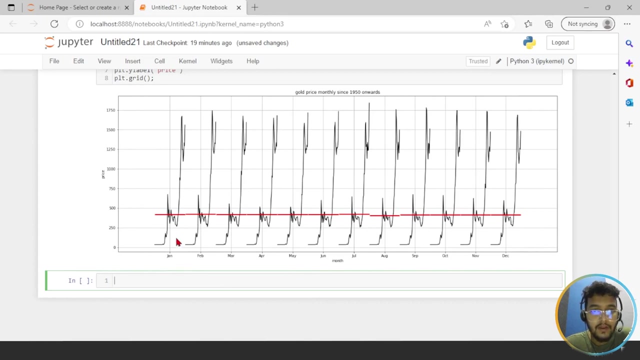 Okay, and pltxlabel month, and pltylabel, the price, pltgrid. so here you can see gold prices monthly since 1950, like for every month, like january, february, march, april, so on till december. okay, we will cover one more thing, one more graph, okay, and many, many more graphs. 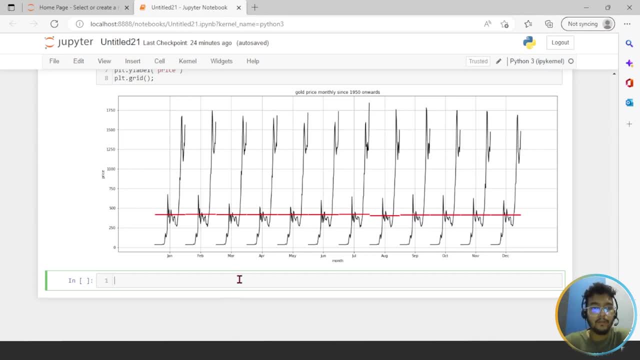 so. so we will go with the next graph, for that i will write here. let's go. ax equals to plt dot subplots and figure size was to 22 comma 8 and same sns dot boxplot x equals to df dot index. dot boxplot x equals to df dot index. 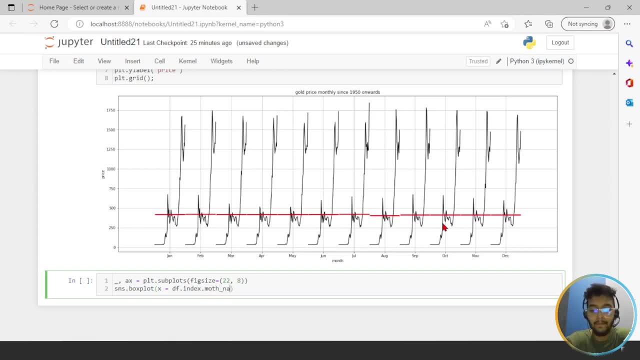 x equals to df dot index. x equals to df dot index. dot month name. okay, then y equals to df dot values. comma zero. comma ax equals to ax. okay then plt dot title: وأ god frog. 妳 will put same title, so i can copy from it. 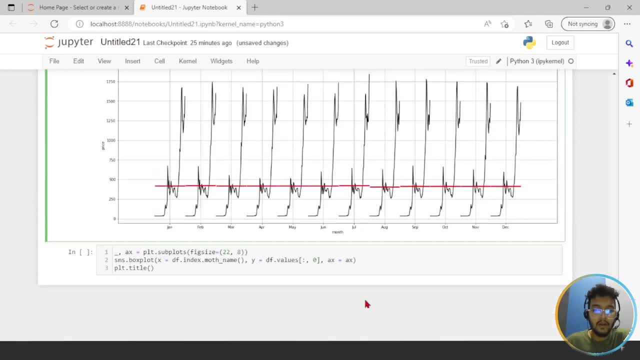 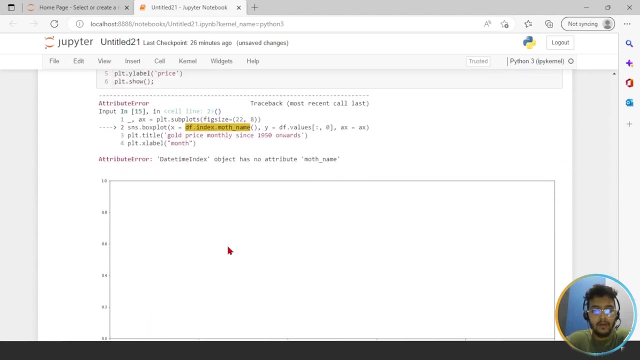 вы đây put same title so i can copy from it here. let's copy from here and paste it here. okay, and pltxlabel, plt dot. xlabel dot y-level price and PLT dot grid. okay, your show. this time let's not use grid. OK, something, i'm going to use month name. 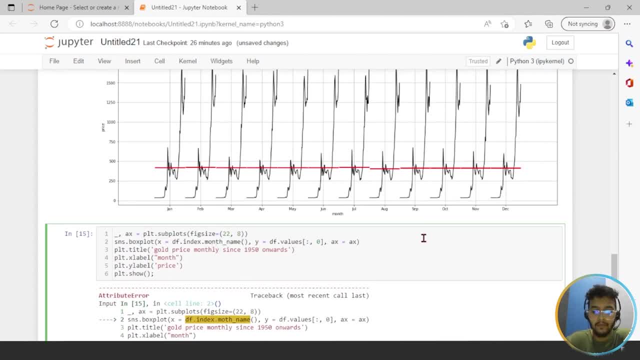 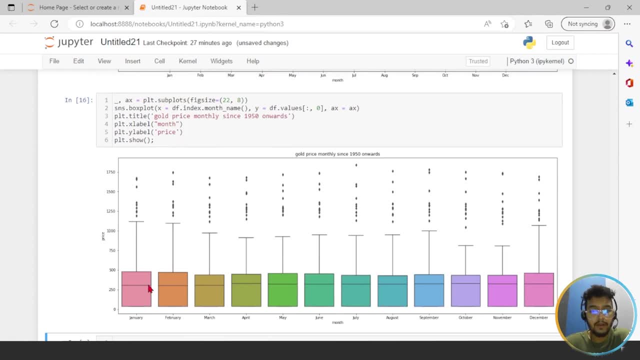 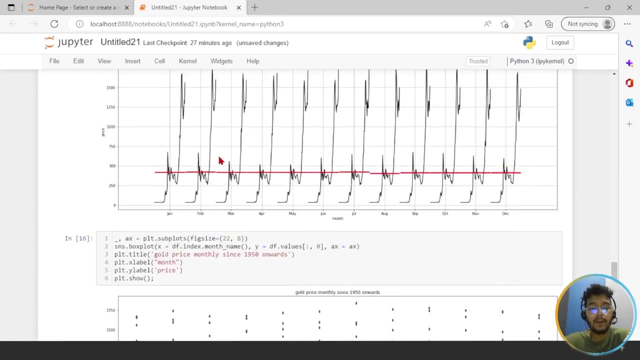 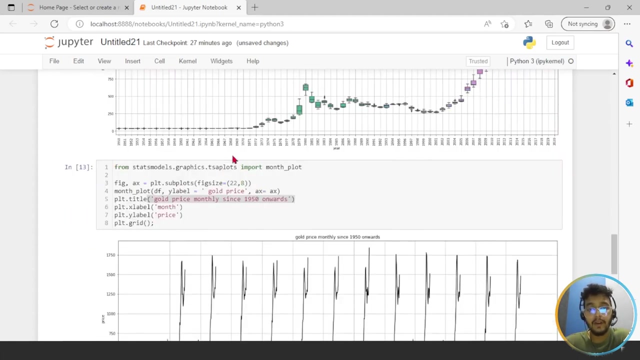 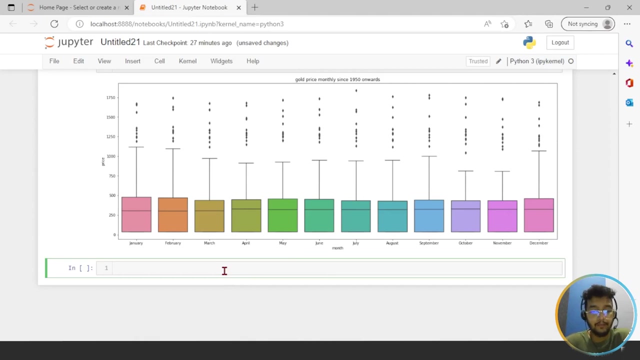 yes, you can see for every month. this is another type of graph, okay, box plot graph. so why we are creating so much graphs? because we are doing EDA data analysis. in this we have to see the multiple, different and different, different types of graph. okay, so moving forward. let's see average gold price per year, like trend since 1950. 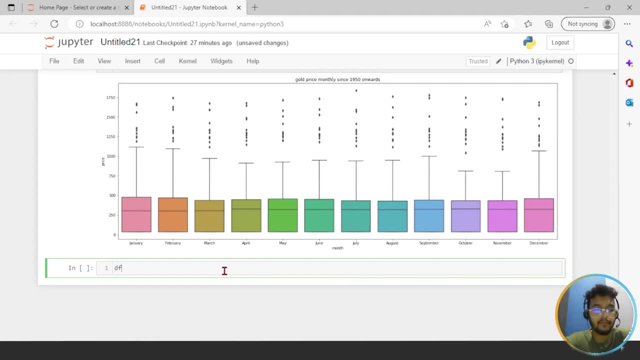 so for that i have to write here df. let's go yearly, let's go some df, dot the sample, sample, then a dot mean df, underscore, yearly, underscore, sum, dot, plot, tlt, dot. title. here i will write average gold price yearly since 1950. or you can write onwards from onwards 1950. 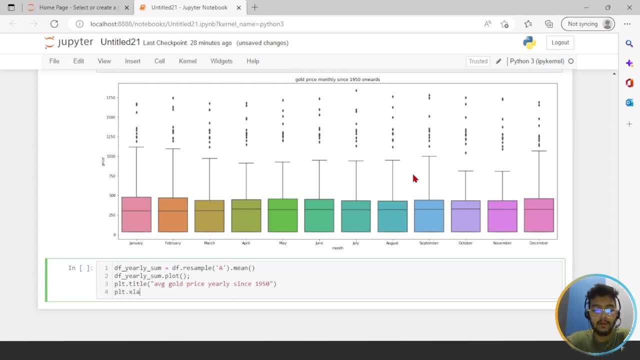 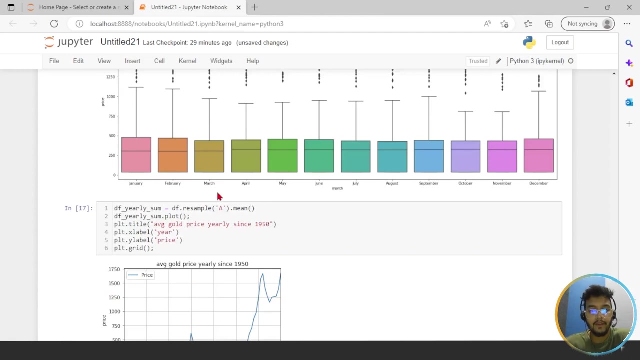 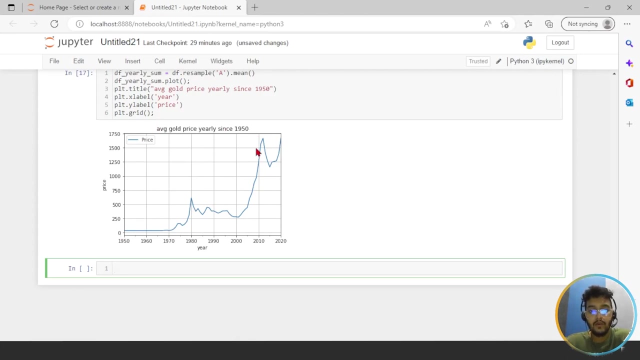 so here i will write plt dot x label here and plt dot y label- ice. okay then, plt dot grid. this time we'll use grid. so here you can see the average gold price yearly since 1950.. okay, this is the chart till 2020, like sometimes up, sometimes down, okay. 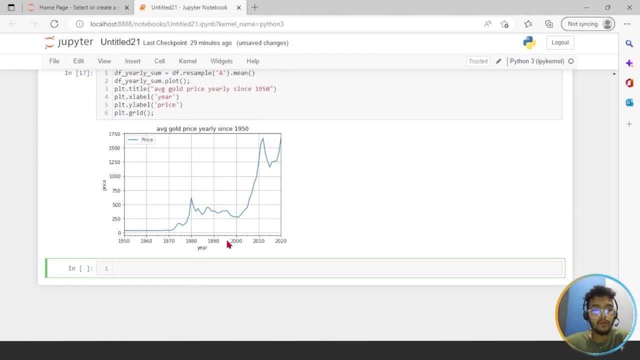 and we will see now, like average goal price per quarter, like trends like since 1950.. so here i will write df dot, not dot, df dot quarterly, like trends like since 1950.. so here i will write df dot, not dot, df dot quarterly. 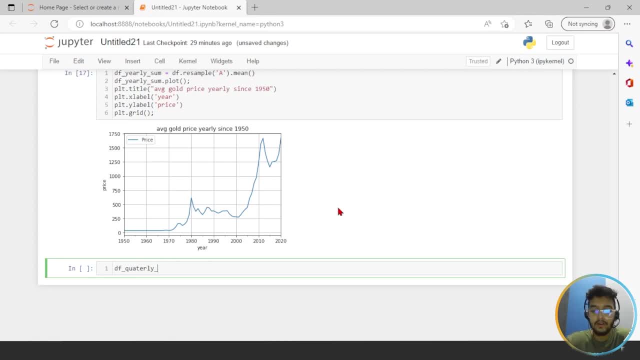 Okay, underscore sum equals to df dot resample quarter q dot mean. move this. then df underscore quarterly score sum dot plot and the same plt dot title. from here here i will write: average good is quarterly, quarterly, okay, since 1950. then plt dot x label. 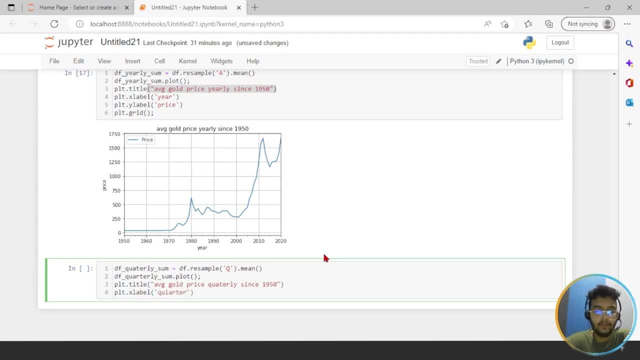 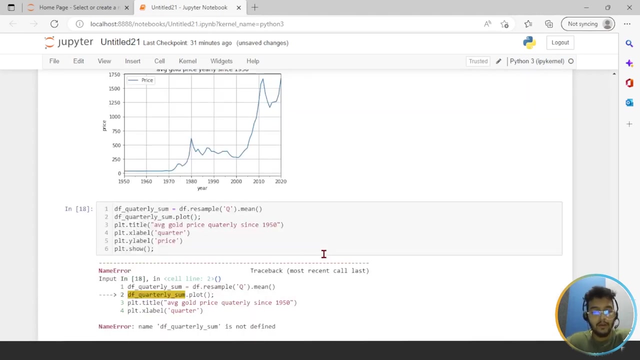 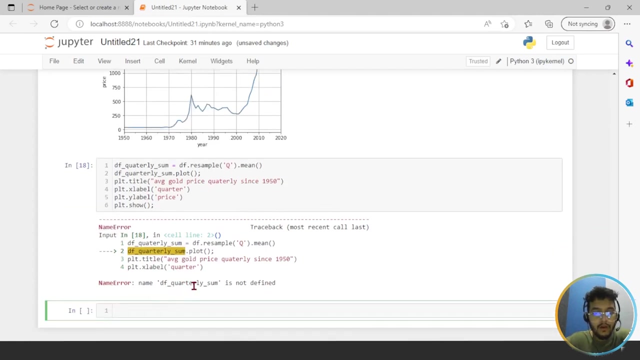 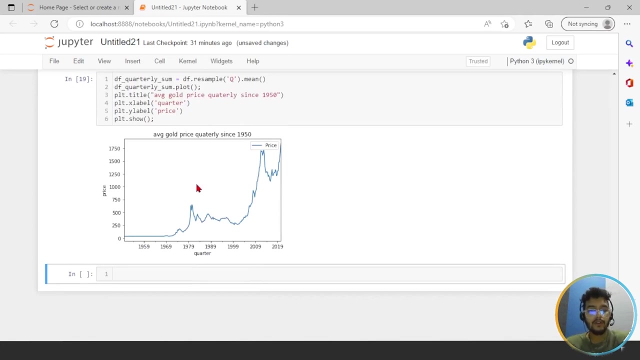 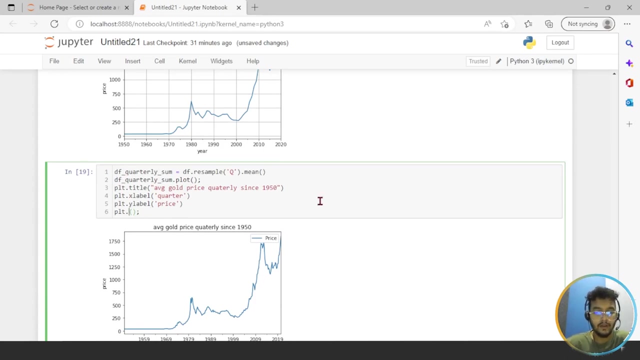 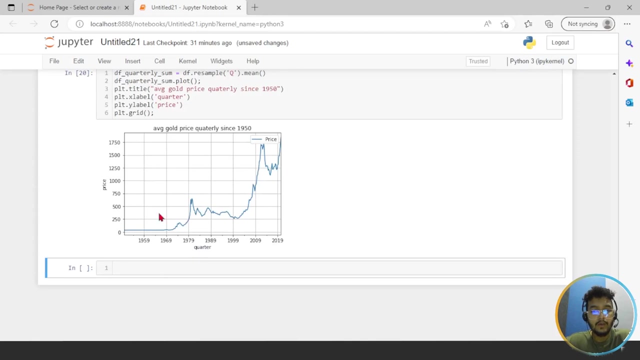 label is now here. quarter plt dot y label is price. okay now plt dot. show this time: okay, df underscore quarterly: okay, quarterly. yeah, here you can see the price prediction. okay, let me set to the grid. only, it's not this. results are not good, so great, yeah. so here you can see the quarterly. 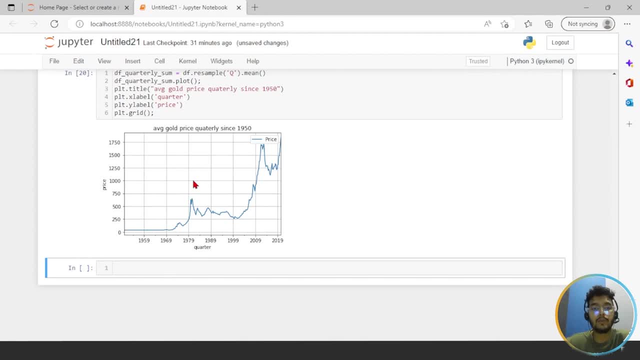 prices prediction. okay, average gold price quarterly prediction. so like moving forward, we will see now average gold price per decade, like per 10 years. okay, so from 1950 only. so here i will write df underscore- decade. underscore sum equals to df dot resample every 10 year. okay, 10 year. 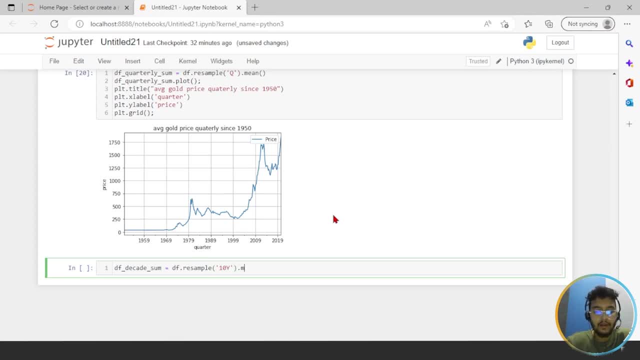 right, dot mean we are writing, mean because we are like putting out average. okay, so df underscore decade, underscore sum dot plot: plt dot title. plt dot title: average gold price per decade since 1950. okay, since 1950. yeah, perfect, so here i will get plt dot. 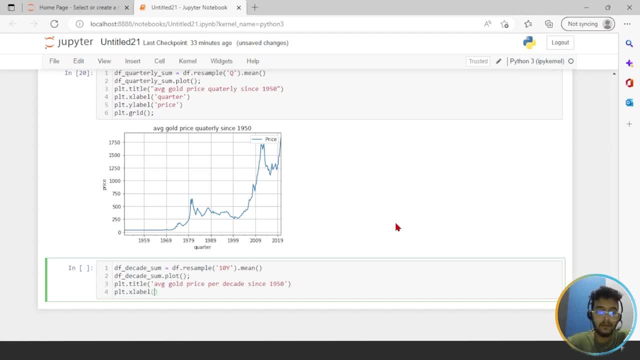 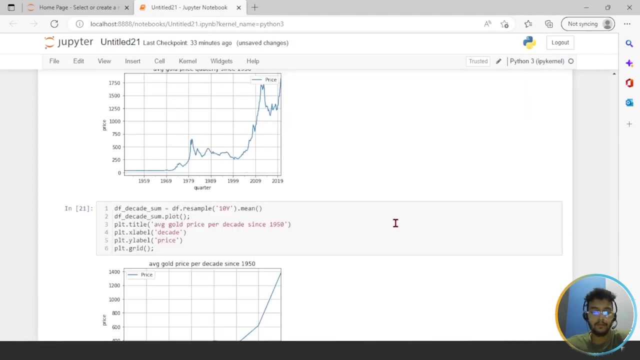 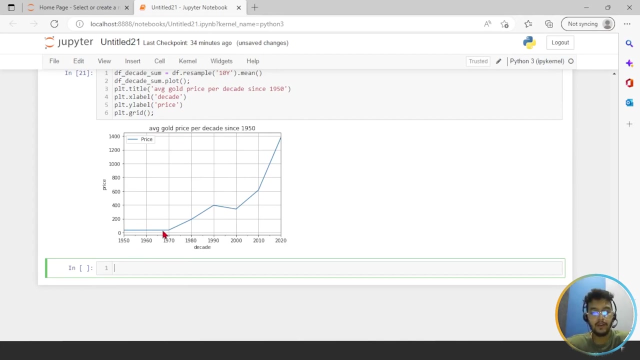 x label, then decade, decade is off, like every 10 year. plt dot y label. plt dot grid. yeah, so here you can see the average gold price per decade, like from 1950 to 1960, like this: straight, then again, straight, then up, then sometimes down, then up and down. okay, every 10 year you can. 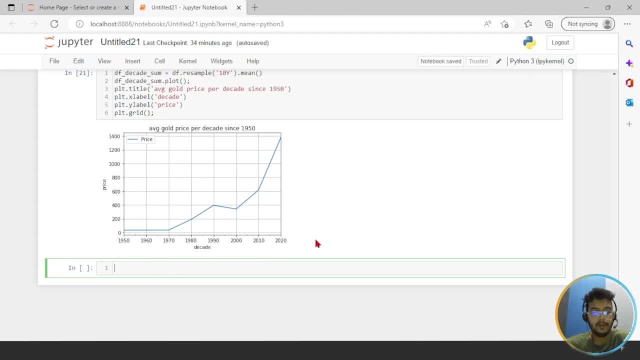 see a 1990, 2000, 2010 and 2020. so moving forward. let's do like analysis in coefficient of variation. the coefficient of variation cv is a statistical measure of the relative dispersion of data points in a data series around the mean. and in finance, the coefficient of variation allows investor to 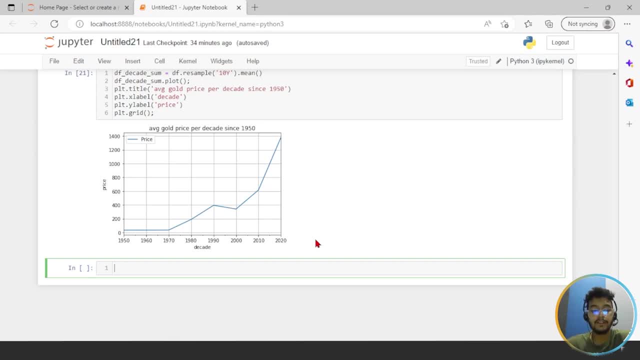 determine how much mortality or risk is assumed in comparison of the amount like amount to the return expected from investors. okay, the lower the ratio of the standard deviation to mean return, the better risk return trade-off. okay, let's like. let us look now the cv values for each year in gold. 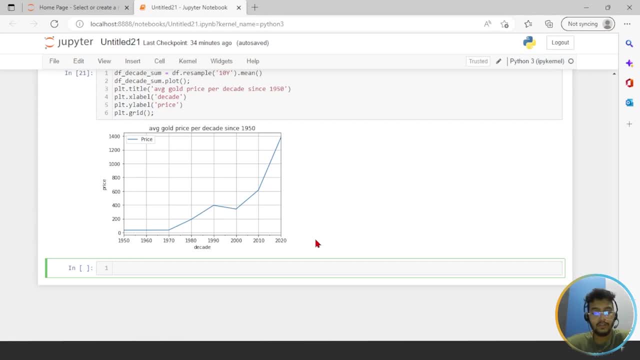 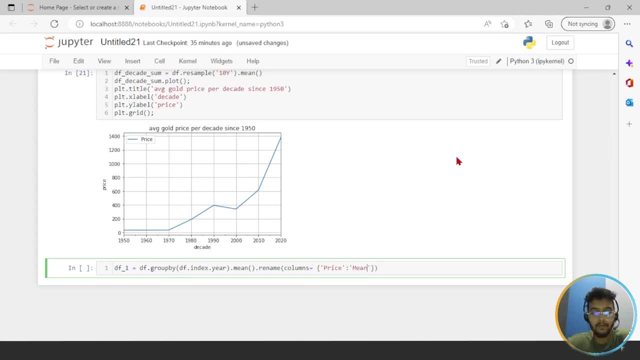 and mean and mean: okay, then again df underscore one. okay, then again df underscore one. okay, then again df underscore one equals to df underscore one equals to df underscore one equals to df underscore one. dot range, dot range, dot range, or what we can do instead of range, we 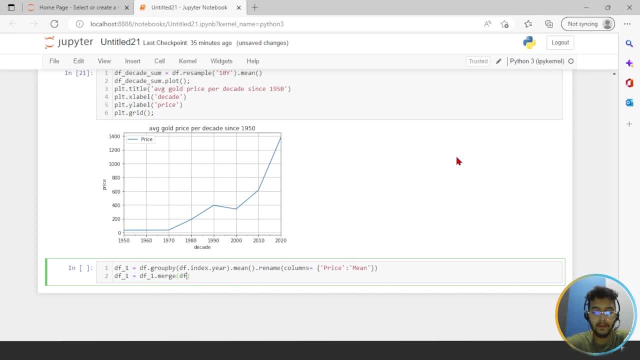 or what we can do instead of range. we or what we can do instead of range. we are going to write merge. are going to write merge. are going to write merge. df dot group by df dot group. by df dot group. by let's go, let's go. 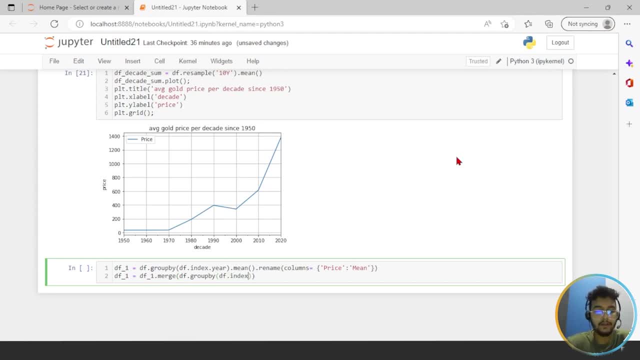 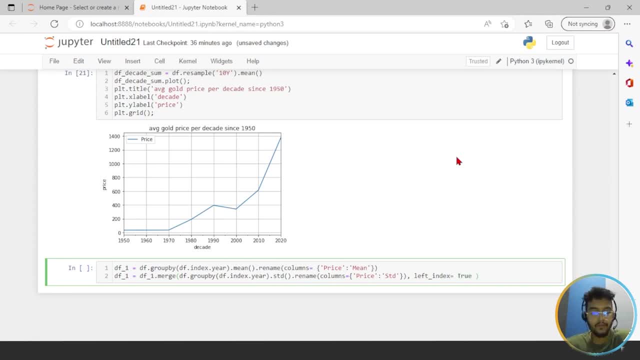 index pursue true. then comma right index: pursue true, pursue true, pursue true. and here df underscore one and here df underscore one and here df underscore one school was to, was to, was to df underscore one was to df underscore one school was to df underscore one school was to df underscore one school. 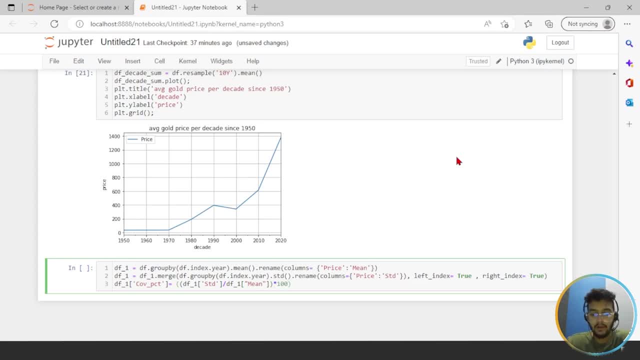 to hundred. like dot. round figure should be like two after round figure should be like two after round figure should be like two after decimal. how much like numbers you want decimal. how much like numbers you want decimal. how much like numbers you want to see to see. to see then: df underscore one dot head. 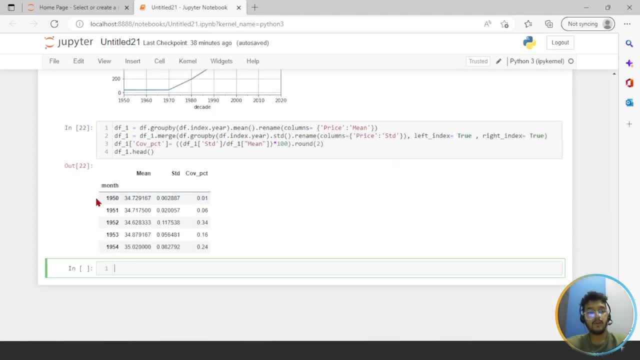 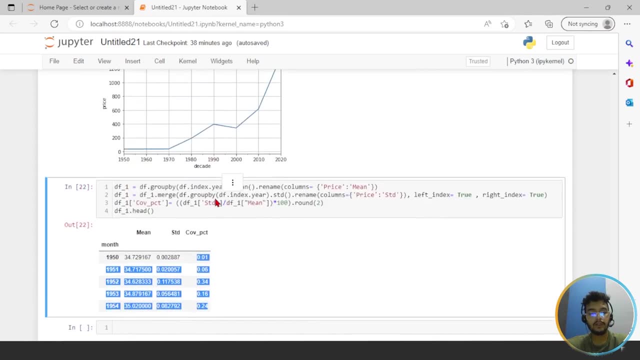 center. yeah, so here you can see for center. yeah, so here you can see for center. yeah, so here you can see. for every year i have mean standard deviation. every year i have mean standard deviation. every year i have mean standard deviation and this coefficient of variation, and this coefficient of variation. 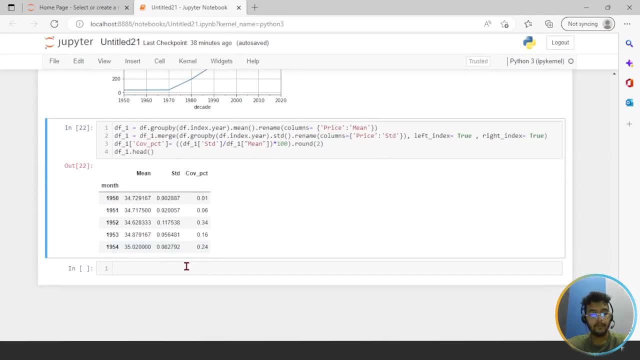 and this coefficient of variation? okay for every year. okay for every year, okay for every year. so like moving forward. let's see the. so like moving forward. let's see the. so like moving forward, let's see the average gold price per year again. average gold price per year again. 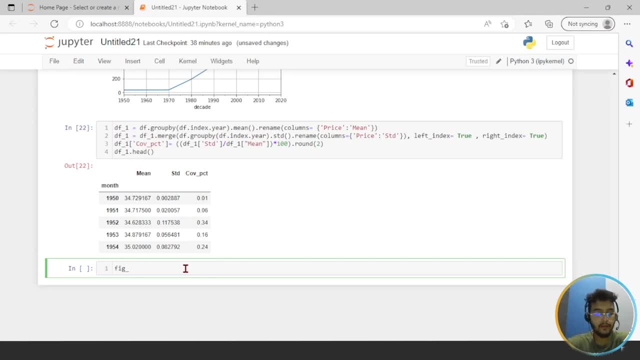 average gold price per year. again, so for that figure, so for that figure, so for that figure. underscore: bigger dot comma ax. bigger dot comma ax. bigger dot comma ax goes to plt, goes to plt. goes to plt. dot subplots, dot subplots bigger size: 15 comma 10. 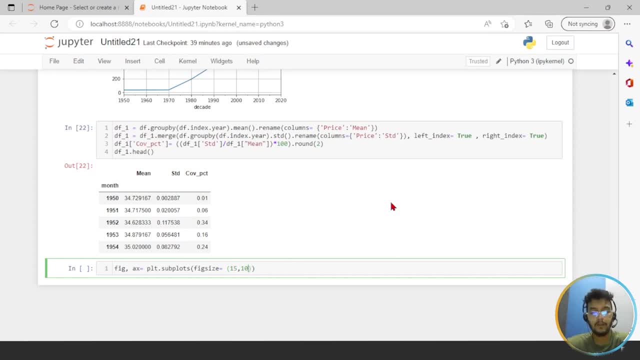 15 comma 10: 15 comma 10. okay, then i will write here: 15 comma 10. okay, then i will write here, then i will write here, then i will write here: df underscore one. df underscore one. df underscore one is: is is cov underscore. 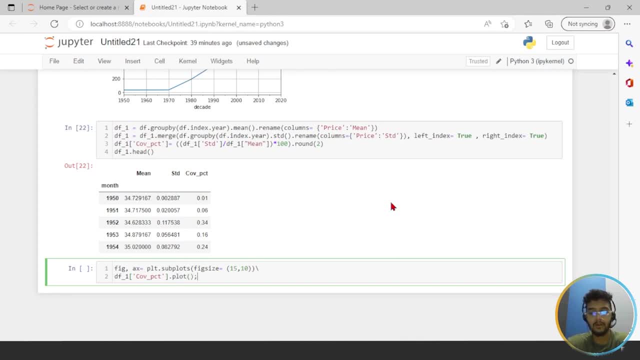 dot plot- elt. dot. title: average average average gold price, gold price, gold price yearly, yearly, yearly since, since, since 1950, from Sousa to 90. bitcoin from Sousa, Coin from Sousa from Sousa. excellent deletion deletion. deletion in percent in percent in percent. okay. 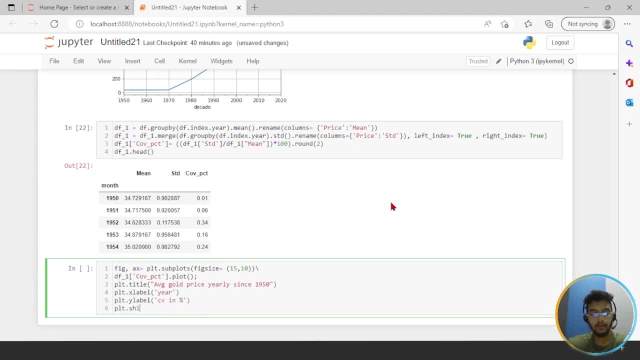 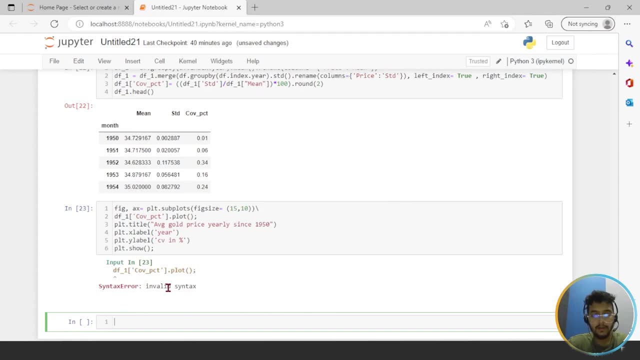 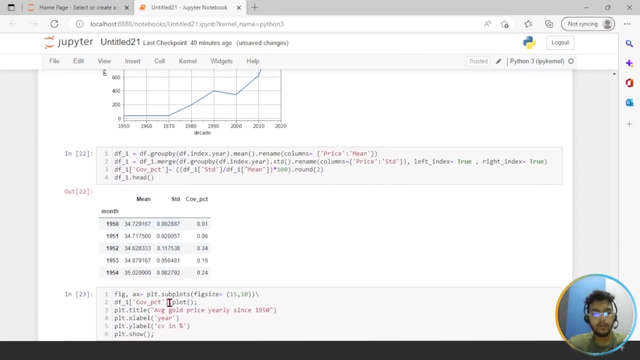 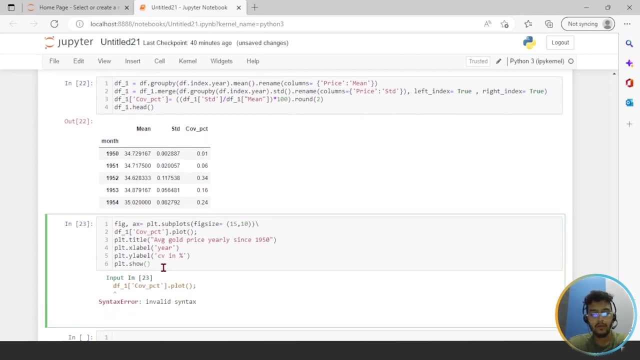 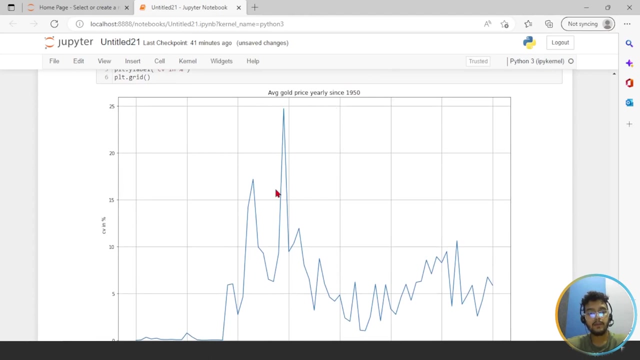 okay, in percent. okay then then. PLT dot. show DF underscore. inverted syntax. COEC script: ECT dot. plot SU: DF underscore one. DF underscore one. write it here: valid syntax: A. So here you can see average gold price since 1950. Okay, This is like percentage. 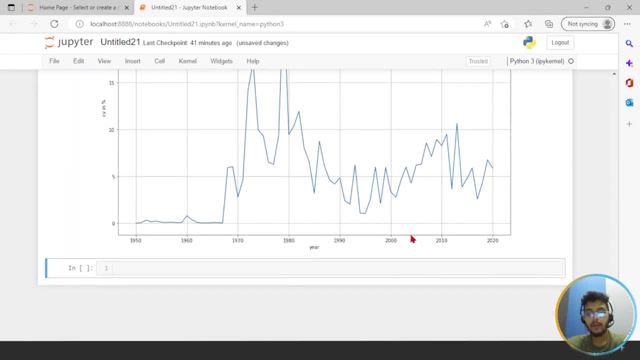 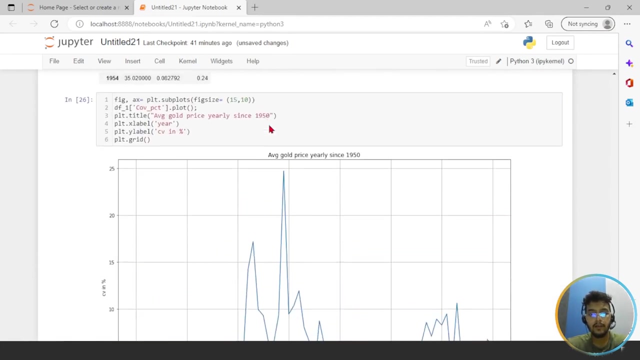 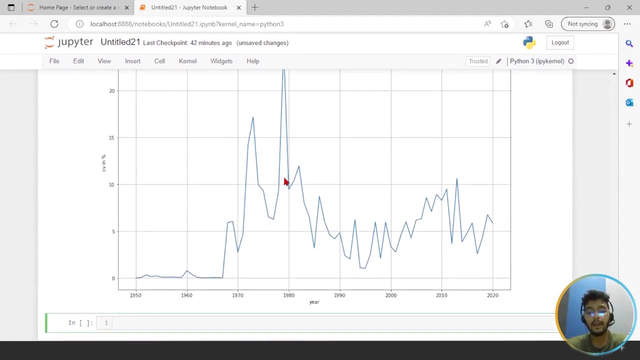 CV in percent. Okay, Like Good, You can see the chart. So the CV value reached its highest in 1978, Like somewhere here. like 1980, 1978, Okay, Like near to 25%, Which could have made the asset as a highly risky. But in 2020 the CV value is closer to 5%. 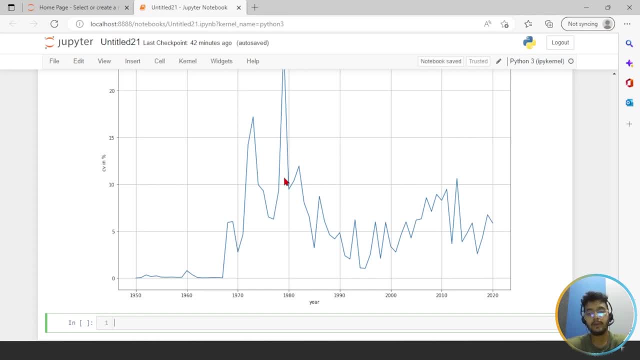 Which makes the asset variable By our good investment. Okay, So Now what we will do? We will do time series forecasting, Okay. We will train model. We will build model, Different, different model. We will train and test split to build time series forecasting model. Okay, So For that, Let me. 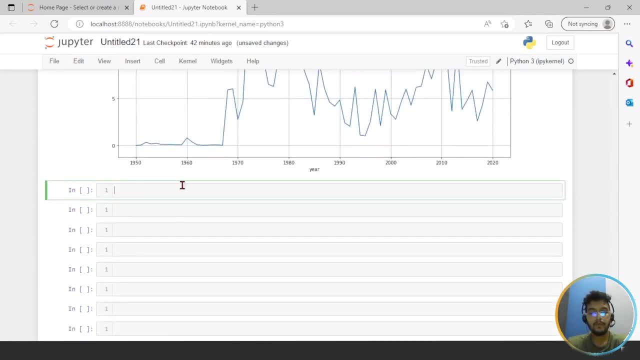 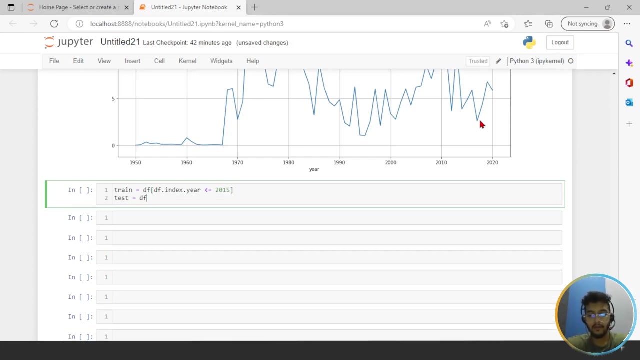 Do like this first. Yeah, So here I will write: train Was to DF- DF dot- index Dot per year. Okay Was to 2015. And for the testing We will write DF- DF dot index Dot year 2015. Okay, For training We are taking till 2015. 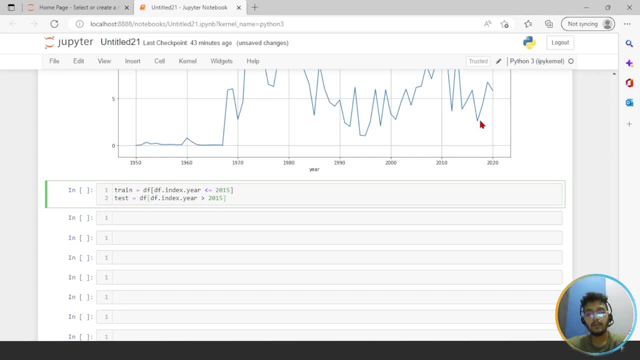 For and For the testing We are taking till 2020, From 2015. Okay, Then I will write here How many columns present in train or test. So for that I will write: print Train Dot Ship And print Test Dot Ship. Press. enter 792 Rows And one column. 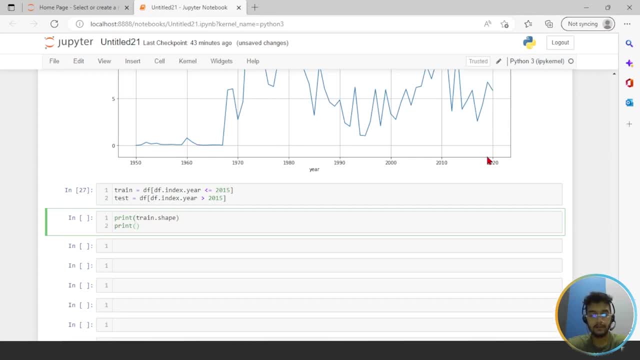 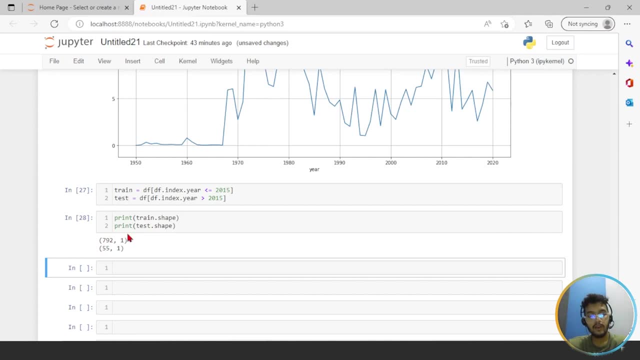 In train Training: For training The model And 55 To test The model: Okay. So We will Do like this. So For training The model And 55 To test The model- Okay. So Now Let's see the training data and testing data. So train Like square brackets. So 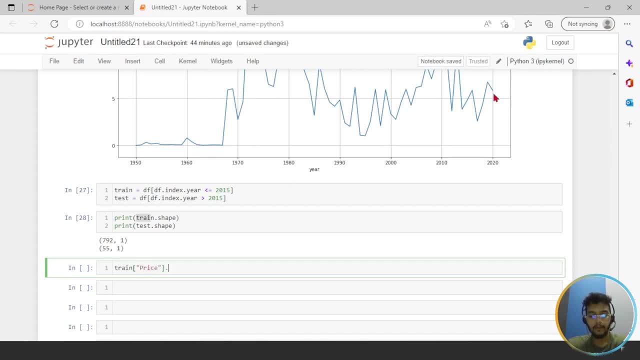 Price Dot Plot. Then Figure size Was to 13 Comma 5, 5, 6, 6, 7, 8, 11, 11, 12, 15, 13, 16, 17, 18, 19, 20, 23, 24, 25, 26, 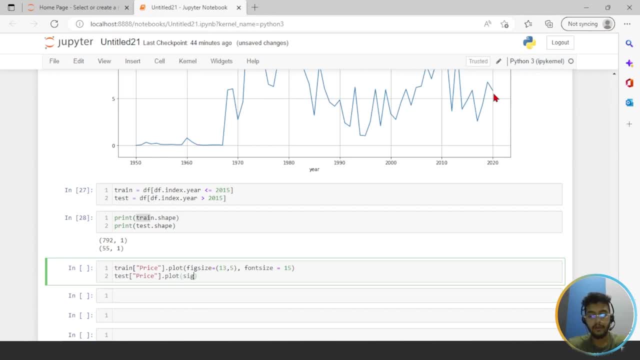 27, 26, 27, 28, 29, 30, 31, 32, 34, 35, 36. let me give same 13 comma 5 font size. should be okay, then PLT dot. let me add great LT dot. great, then PLT dot. agent. 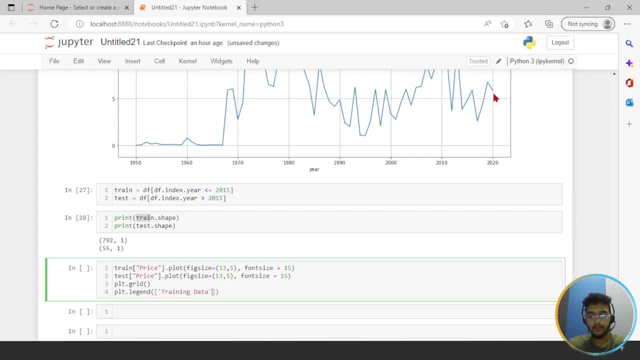 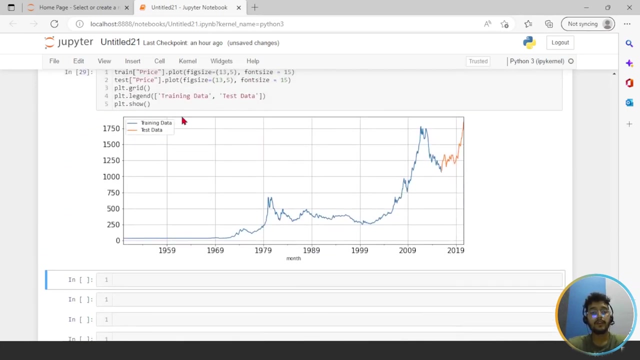 training data, comma test data. okay, then the LT, or so I will tell you what the legend is. okay, so here you can see the training data in blue and the testing data. okay, this is known as the legend, this, this portion, and yeah, so here you can see month wise. 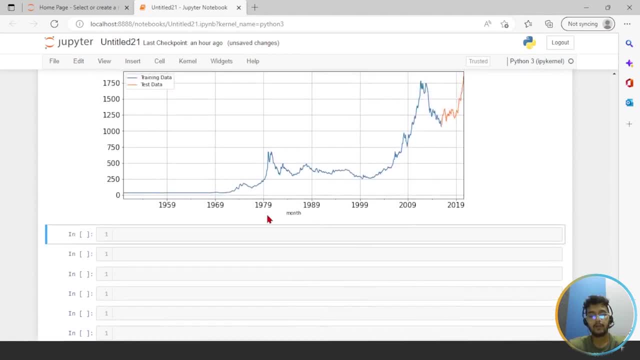 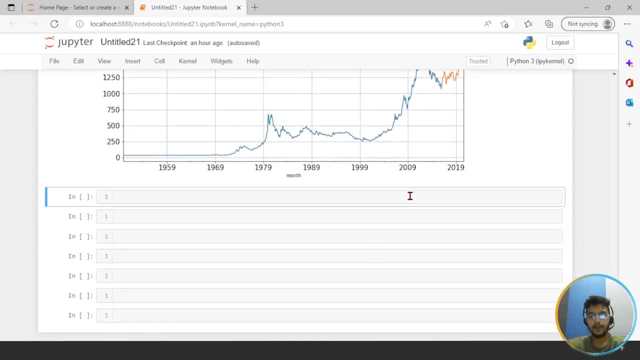 okay, till 2020 and from 1950. right, these are the prices and this is the chart. so, moving forward, let's do model formation now. okay, we will do two models: lineal, linear regression and the name base one. okay, so well, first we are, first we will go from linear regression. for that I will let 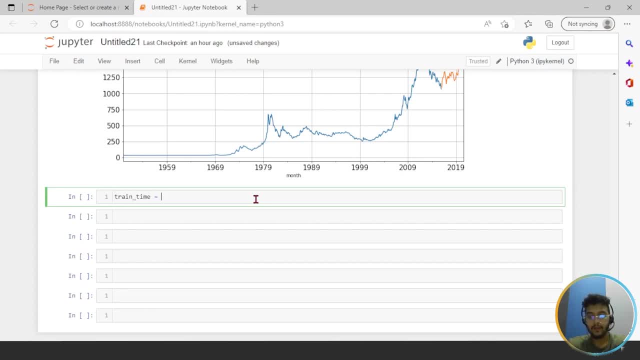 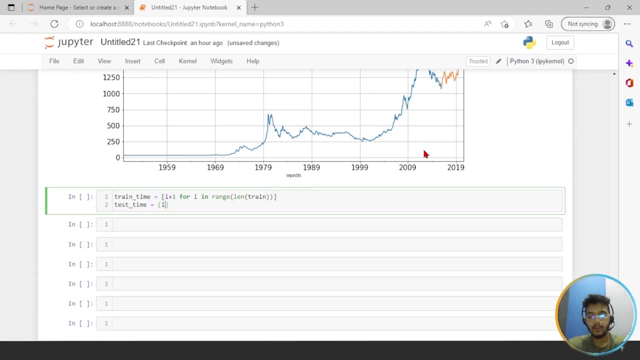 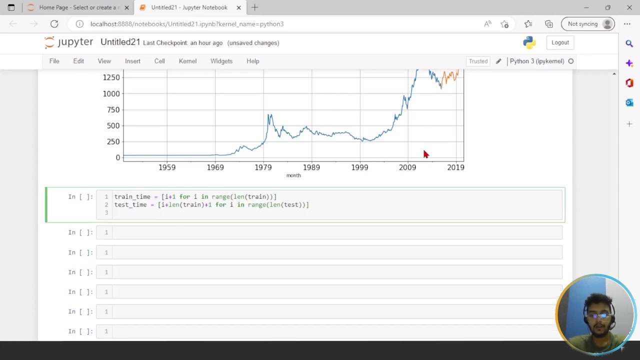 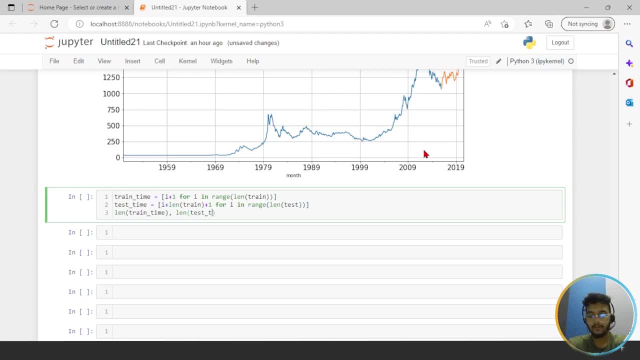 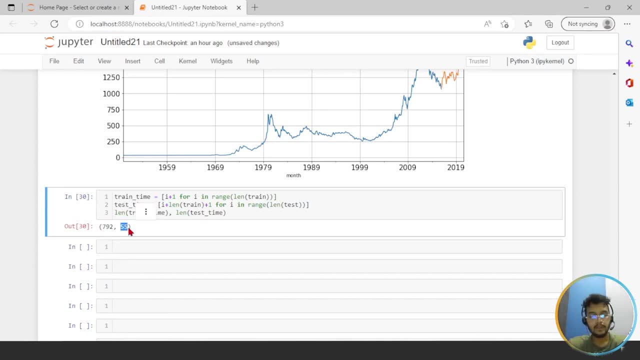 oh, my length should be tested. oh, my length should be tested. a center: okay, this is the training and this for the testing: 792 rows and here 55. a center: okay, this is the training and this for the testing: 792 rows and here 55 게. 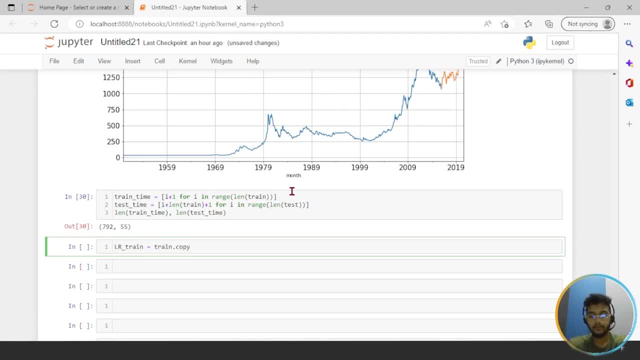 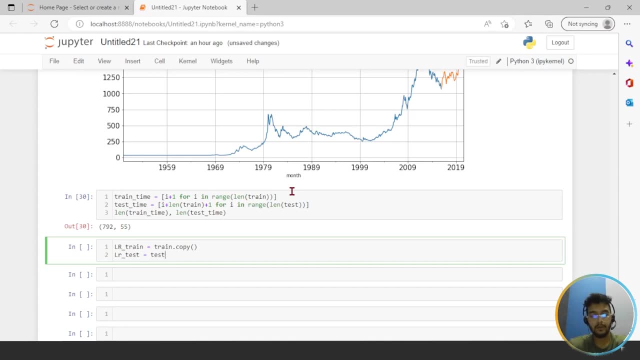 and because to make a copy, can we test it? which is thisgrave up here a center? there's all I am going to show for this test. this is engineering начал underscore. test equals to test copy. dot copy then lr. okay, so lr. train time equals to train time. 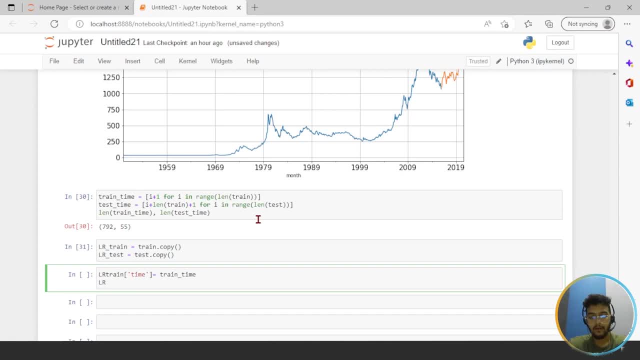 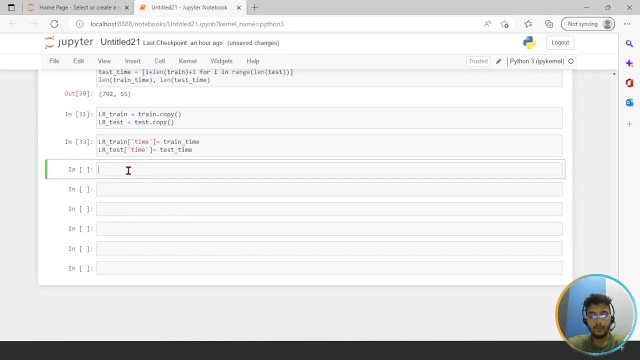 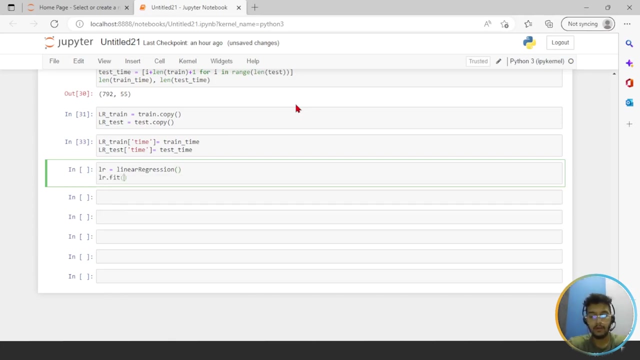 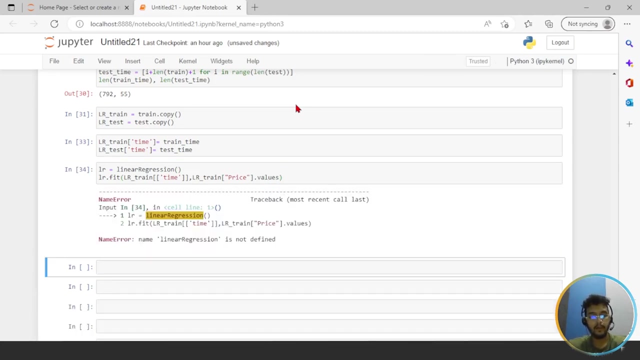 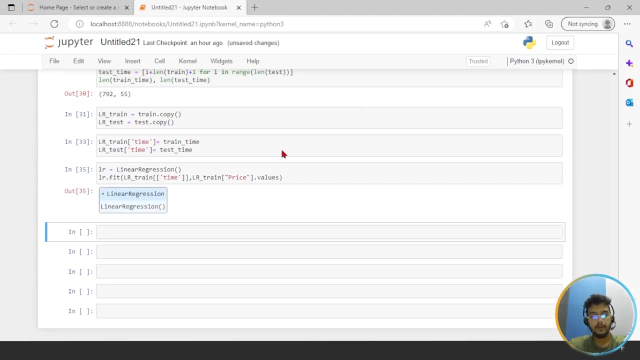 okay, and lr underscore test time equals to test time. okay, underscore is yeah. so here i will write: lr equals to linear regression. dot fit to the model because lr train and for the time la la, underscore train, ice values. linear regression is not defined. okay, my bad, l should be capital, yeah. 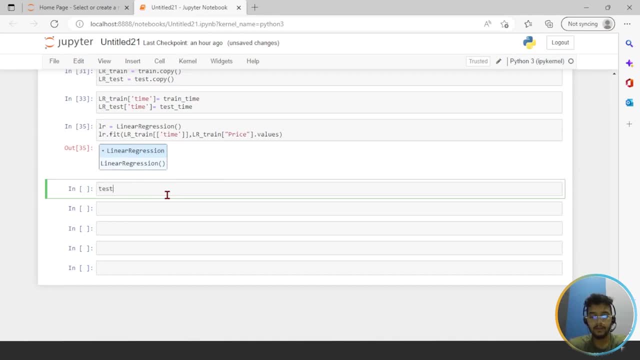 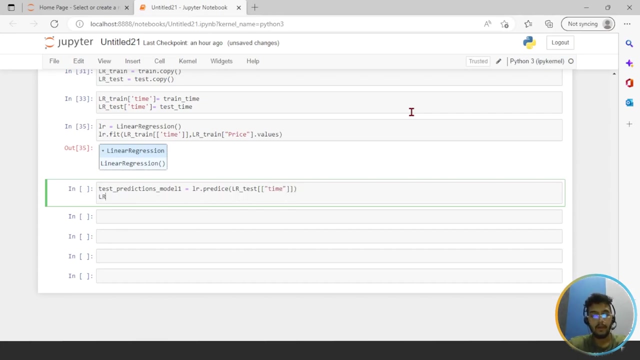 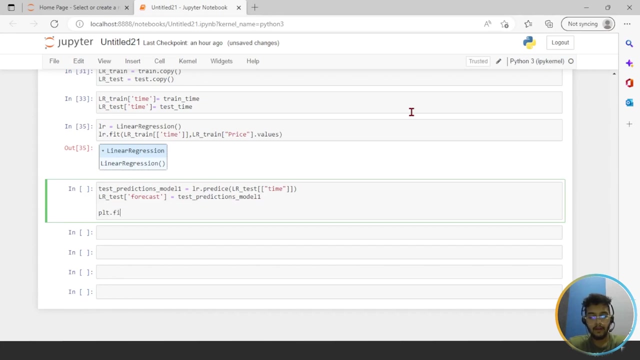 so now see the graph. so test underscore prediction, let's go model one. question lr dot predict. lr underscore test time. lar underscore test. first question: test underscore predictions, let's go model one. okay, let's create the graph figure. figure size should be: let's do 14 comma six. 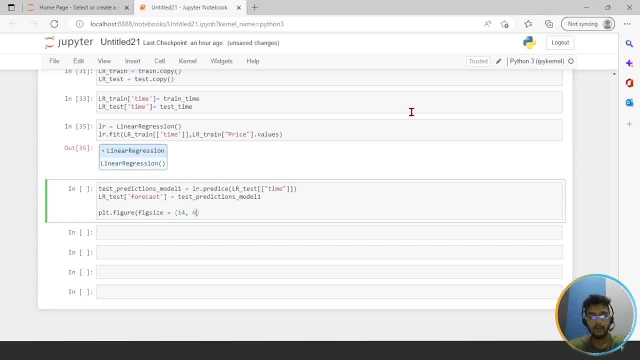 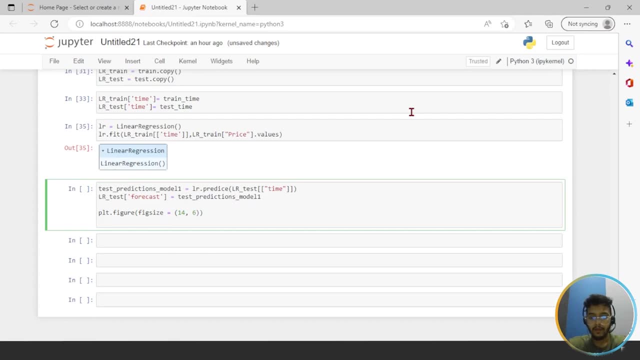 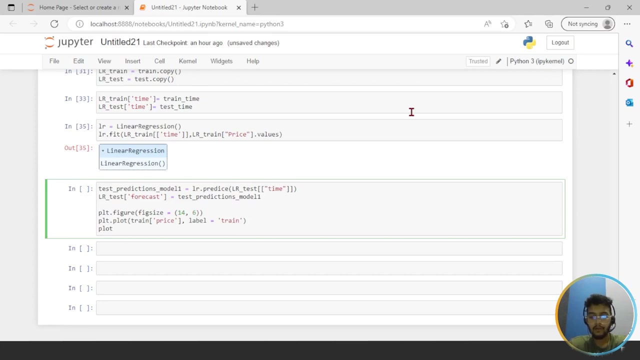 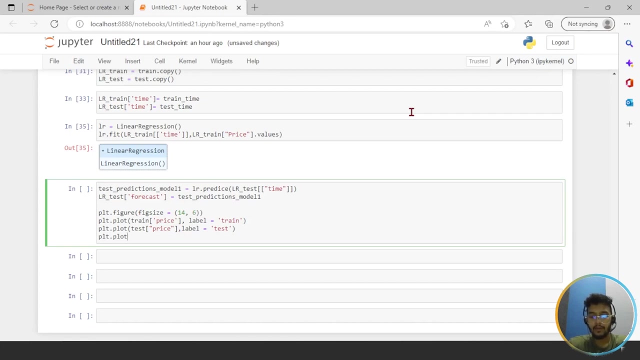 and let's do the next thing. let's say: we see that we've got. our value is like this: let's see three, two, then plot pltplot. test price label equals to test pltplot. then lr train or tests forecast label equals to regression on time. okay, regression on time. 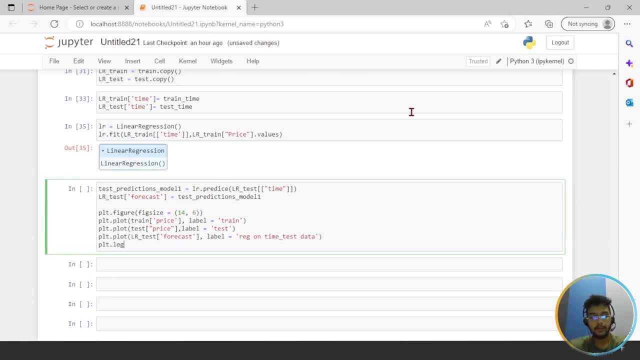 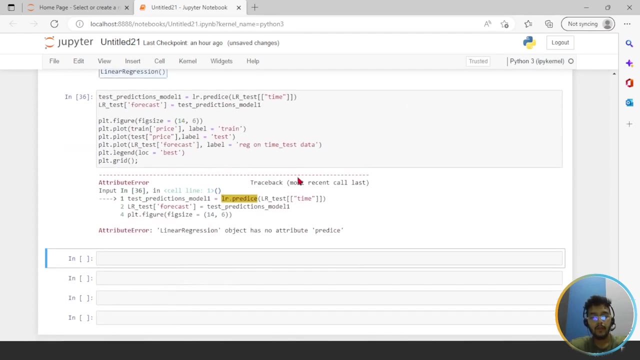 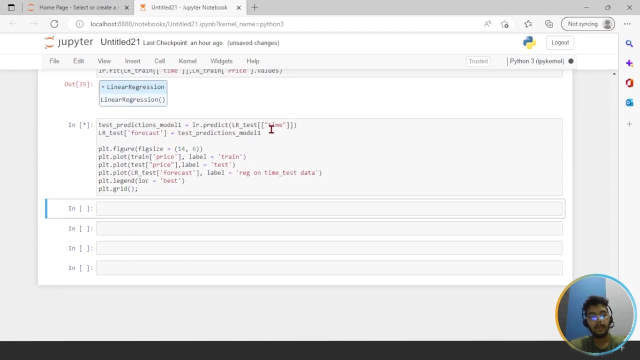 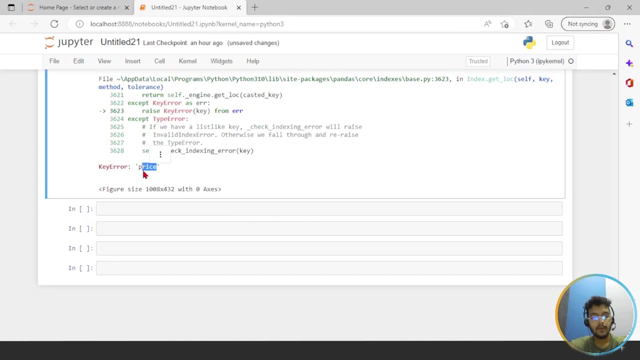 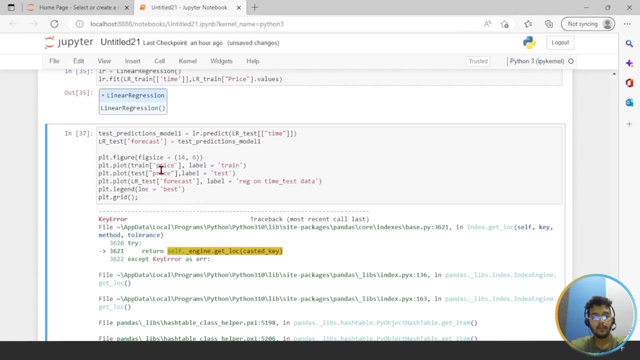 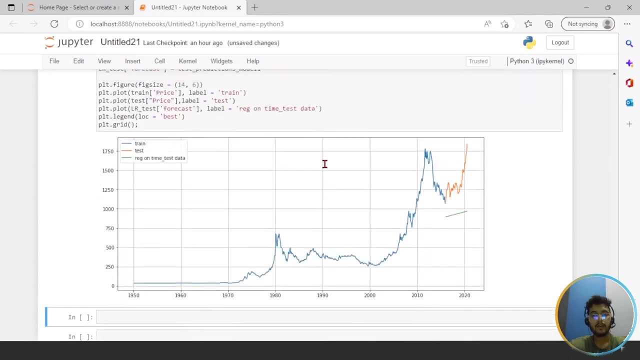 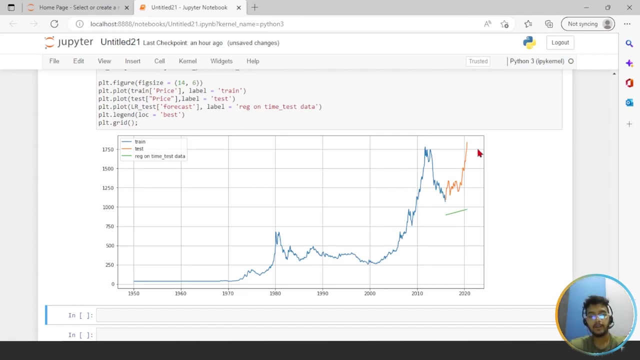 then again pltlegend hello seek equals to past pltedit. press enter. okay, loading one more error price. okay is the price. so here you can see regression on time test data: is this green one and this training data and the testing data. okay, let's find the map now. so for this, 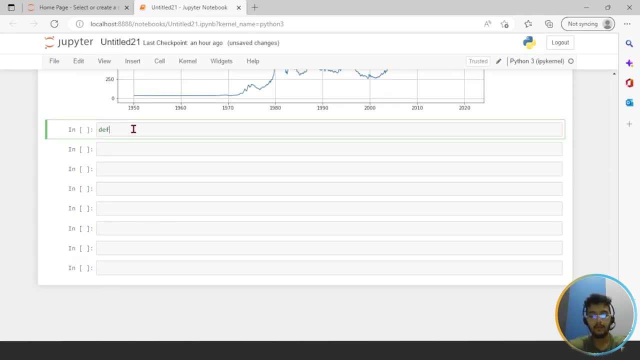 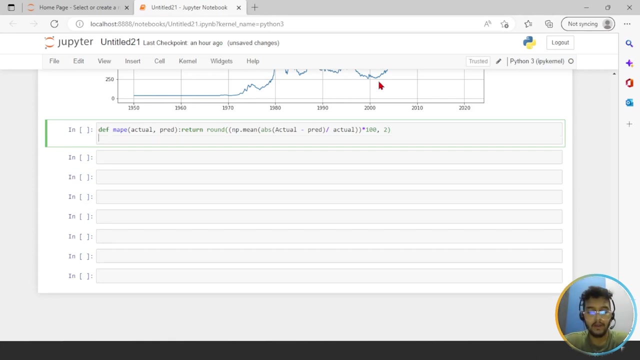 right here: def map, then so target, by then return, say return, return account, pmean, abs, actual action. so I Hundred Comma two, okay, Or to give you yeah. So for for getting the map you have to write a map underscore Order. Let's go test, it goes to me. 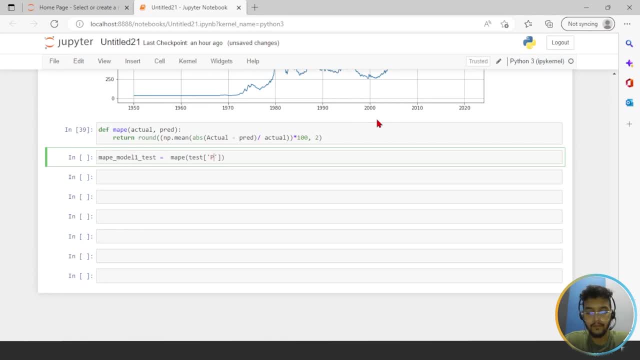 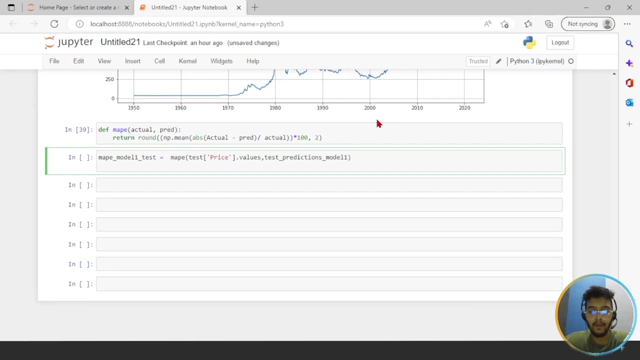 Just Eyes Or Values. Comma test, underscore Action, School model one. okay, then print You: You Is percent three Or three F, Then here every percent. If model You One underscore test, One underscore test, One underscore test, Comma Was a ditch, Was a ditch, Was a ditch. 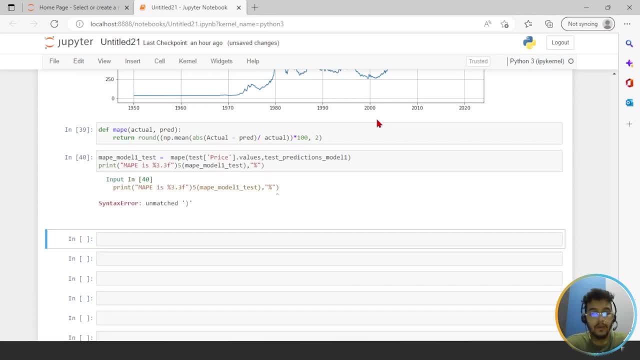 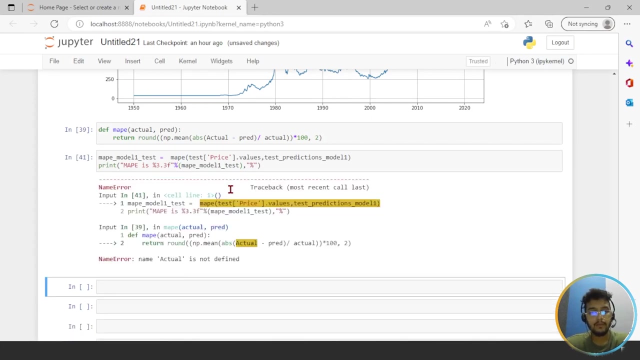 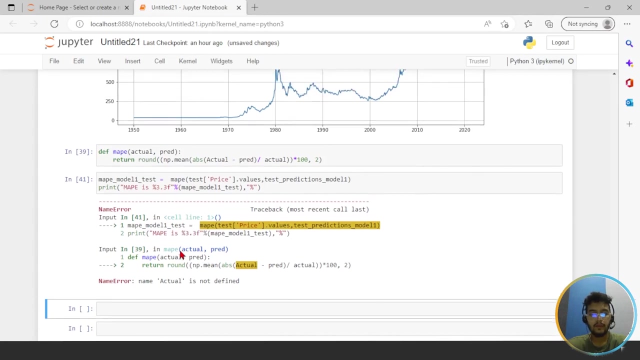 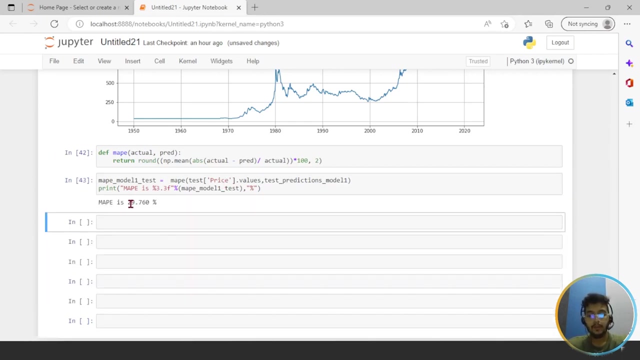 Let's enter. Let's enter Next. Okay so, model one: test. Model one: test. Model one: test Test Values Values Test Test. Model one: Model one: test karena Girls, Yes, yes, As on May be here, you can see twenty nine points and it's just as you know. 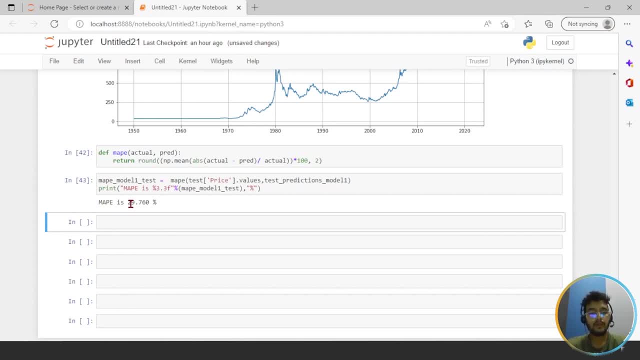 So you are a bit confused, like what is maybe. maybe is a major of prediction of accuracy of a forecasting method in a statistical model. Okay, is a major of prediction accuracy of forecasting method in and now results. equals to pddataFrame test map in percent map underscore model1. 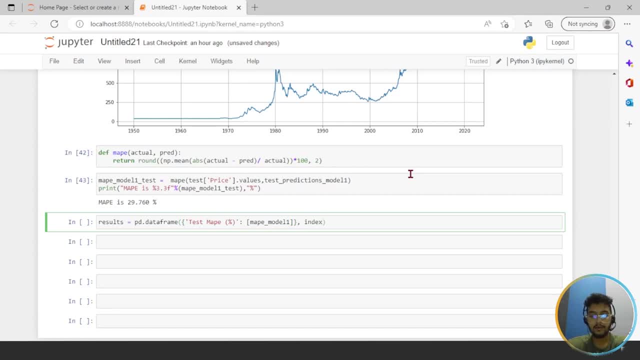 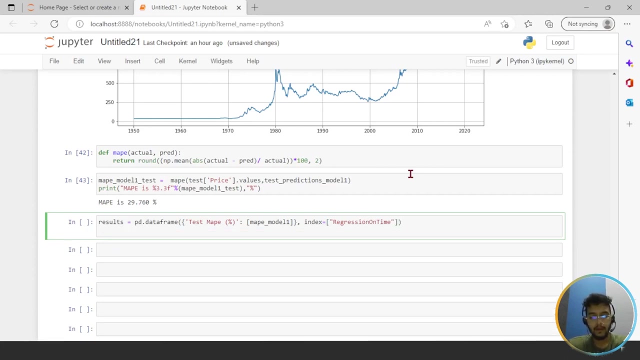 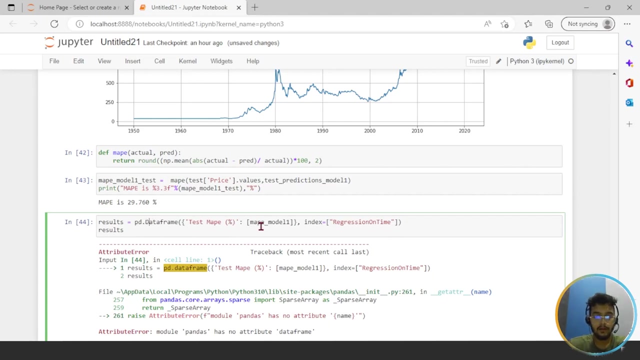 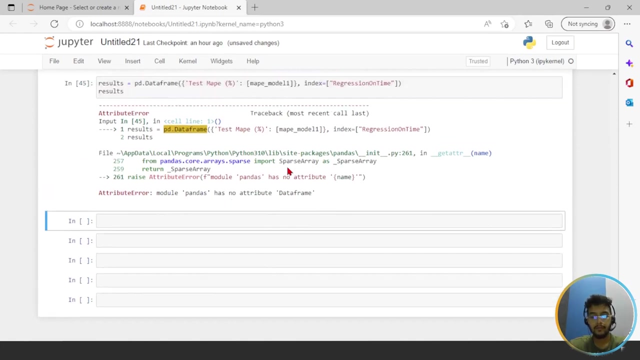 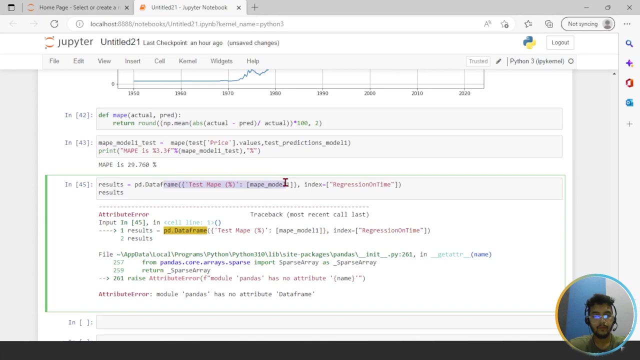 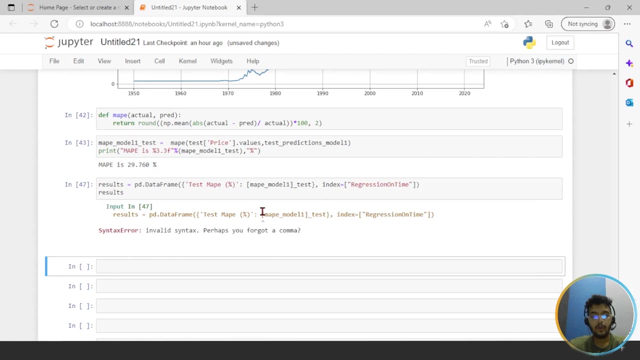 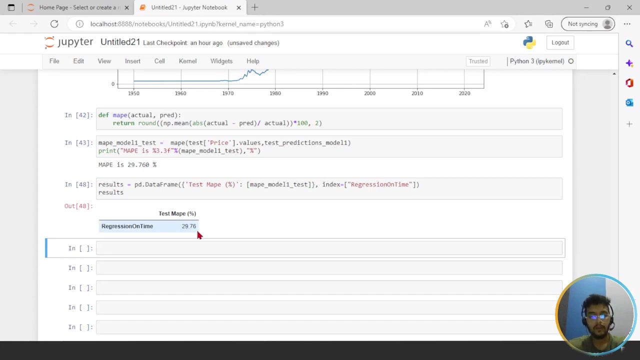 comma index equals to regression on time. then I will print the results. d should be capital module. pandas has no attribute dataFrame. ok, model1 is not defined, let's go test. well, it's in there. perhaps you gotta forget a comma colon model1. ok, here you can see the test map: regression on time. 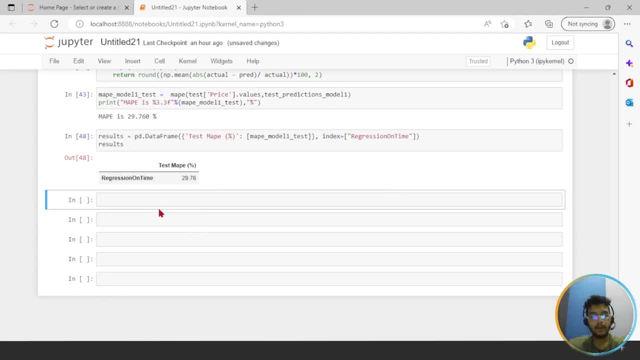 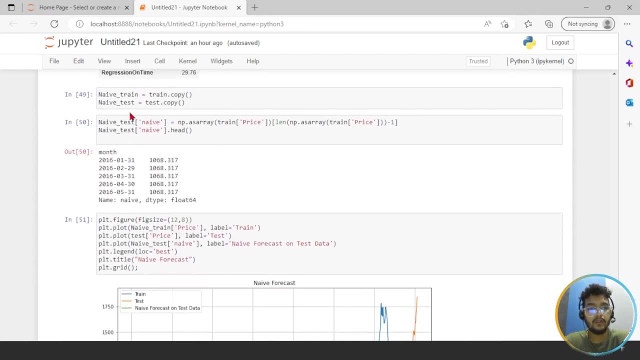 so let's do with the name. now we have to perform the same pattern. so what I will do, what I will write the code and get back to you. ok, I'm done with the code. so here you can see I have same pattern, train and test copy. 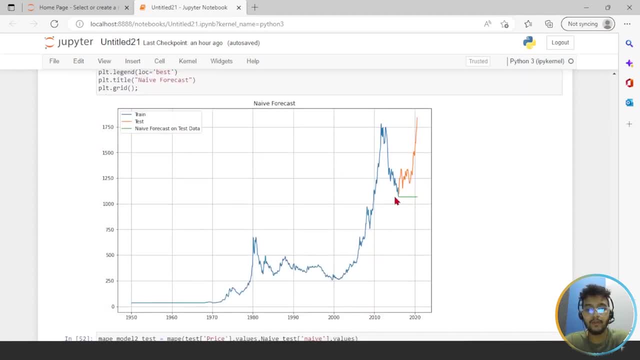 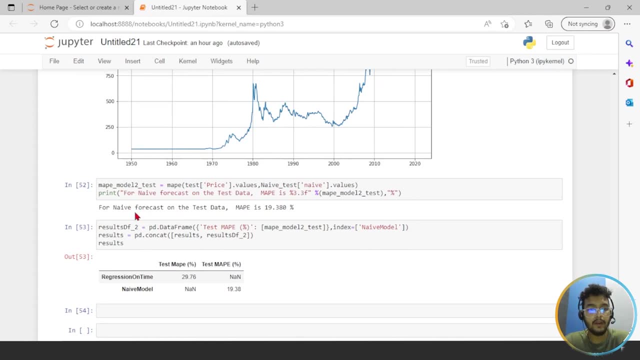 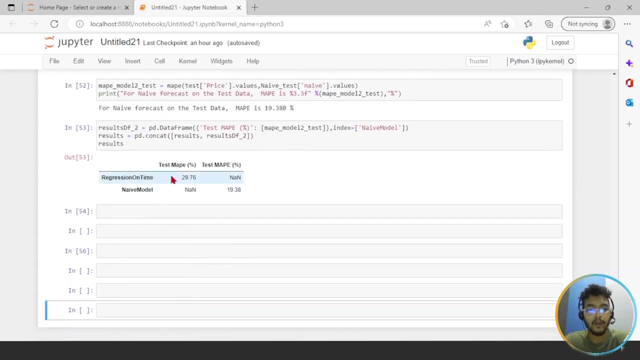 and this is the name forecast on the test data. so this is the line and this is the training and this orange one is testing the same we have got may like 19.380, ok so, and regression: is this the name model? so what we will do, we will create now final model of ours. 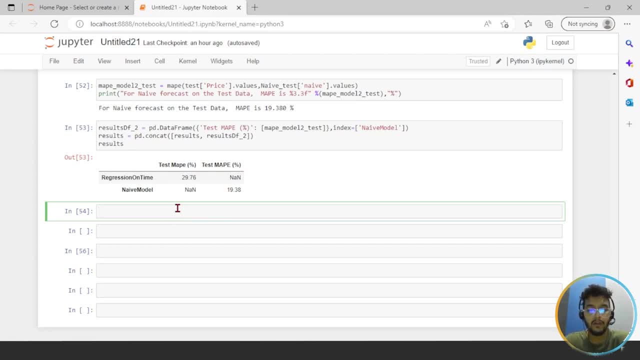 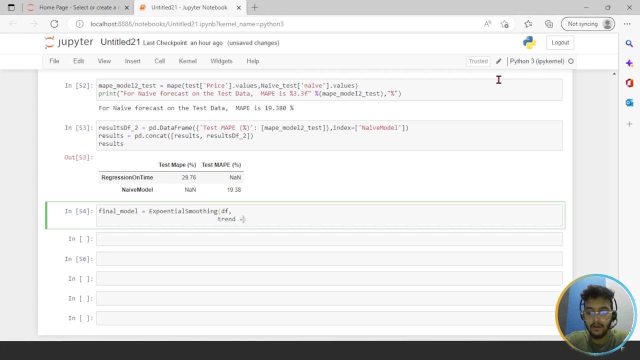 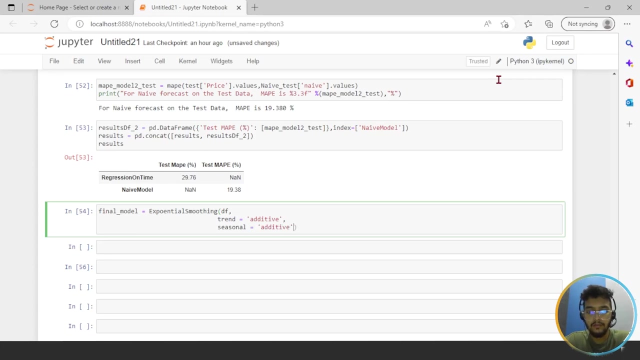 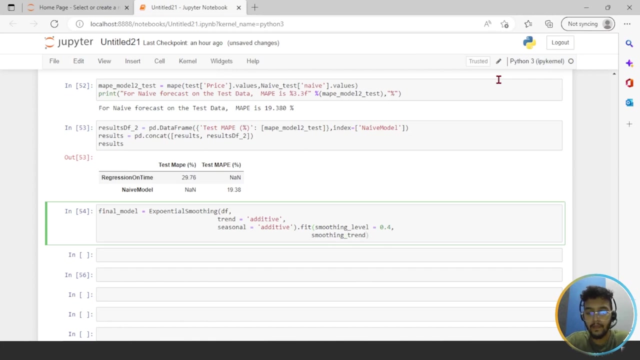 ok, we will forecast. final forecasting will do for that. I have to write final model. equals to exponential smoothing- ok df comma and equals to relative comma. seasonal equals to additive comma. fit smoothing level equals to 0.4 comma. smoothing trend equals to 0.3. 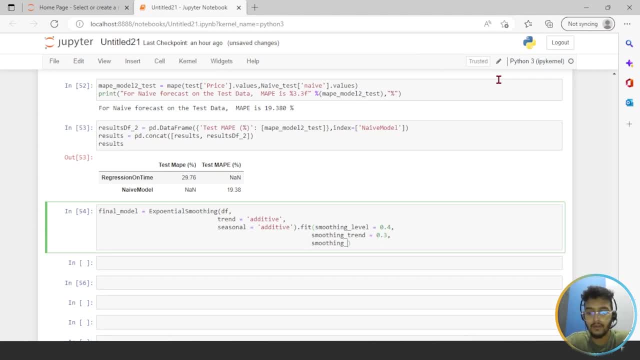 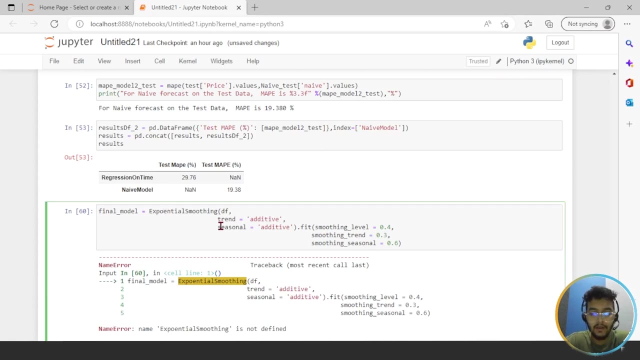 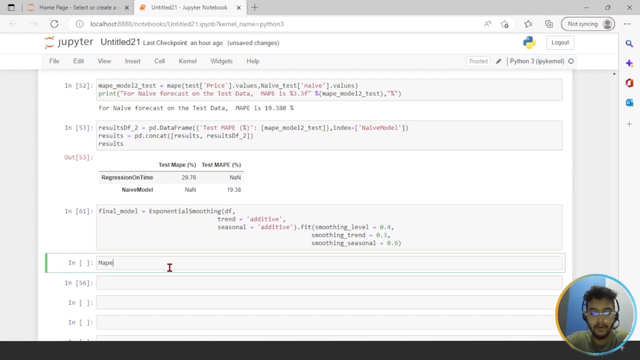 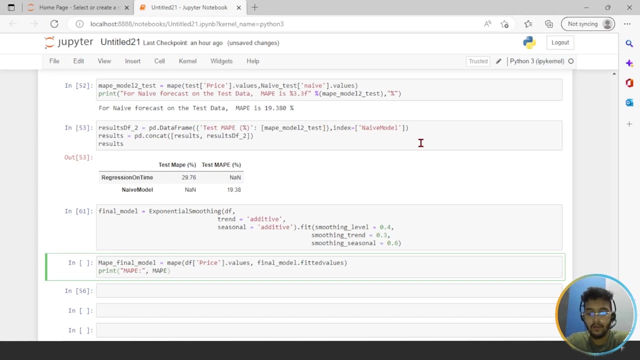 comma smoothing: seasonal equals to 0.6. ok, press enter exponential: exponential: so map. so final underscore model is equals to map. like df size, dot values, comma final underscore model: dot fitted values. then print map: comma map score, final underscore model: ok, so map is 17.24, which is quite good. 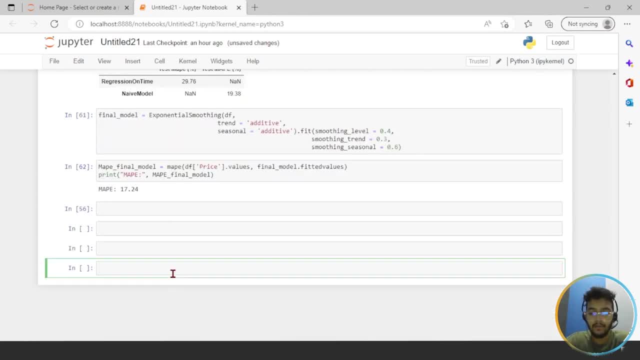 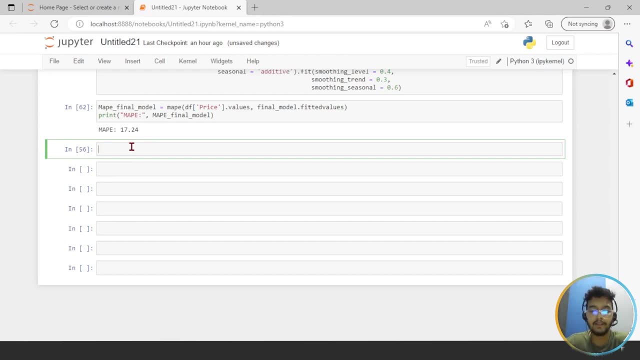 for the final model. ok, so getting the prediction for the same number of timestamps at the present time in the test data. so I will add here predictions: predictions equals to final underscore model dot forecast steps equals to length dot test center. now we will compute 95% of confidence interval for the predicted value. 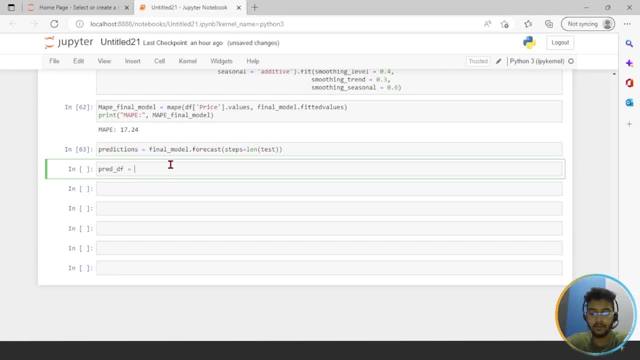 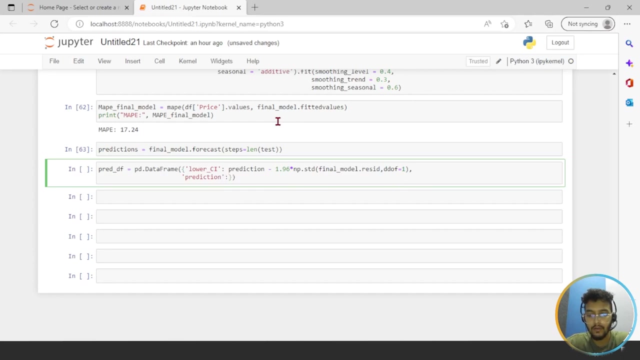 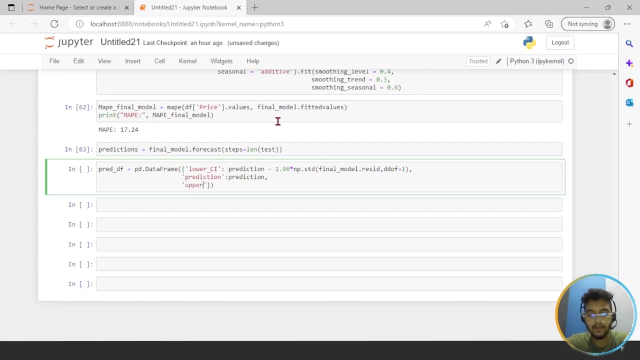 so dkf equals to pd dot data frames. data frames than lower ci. i prediction 1.96 into np dot standard deviation of final model. dot two column, two down maximum. okay, and comma right here. prediction prediction: okay, then upper ci prediction plus 1.96 into dot standard deviation, the same final model. 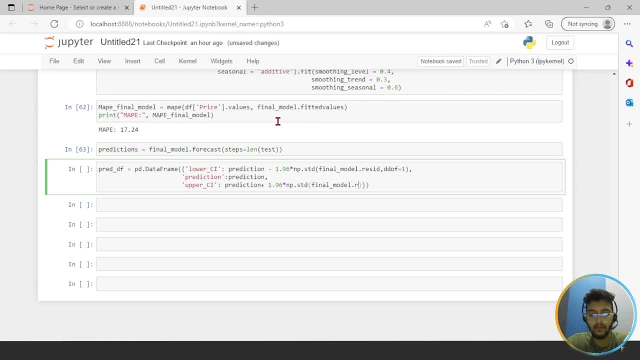 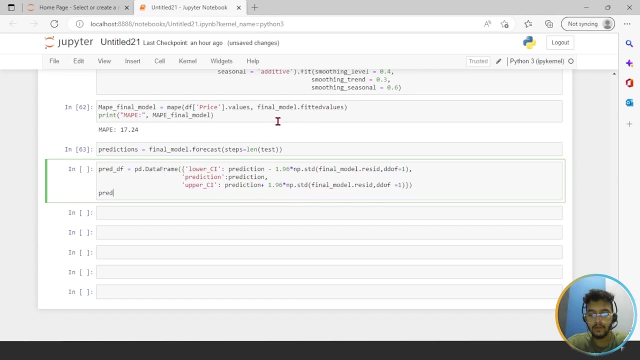 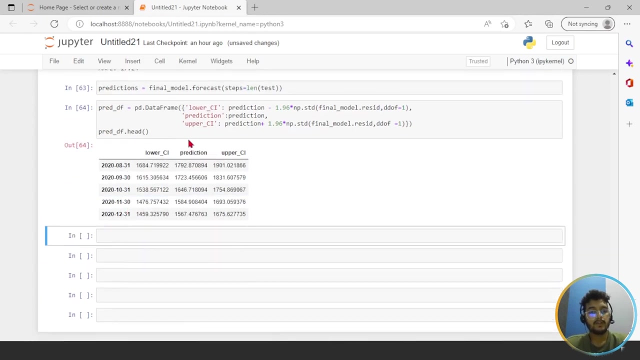 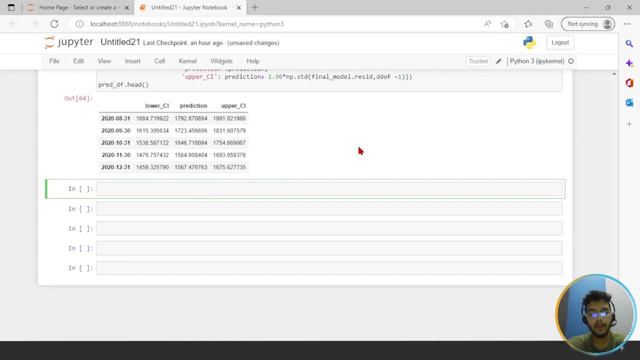 or so one. okay then prediction underscore: df dot at: so this is lower ci prediction and the upper ci, okay, how much it will forecast. or now, at the end, at the final state, what we will do. we will plot a graph, okay, forecast graph, along with the confidence band. so for that, x is equals to df dot. plot label was: 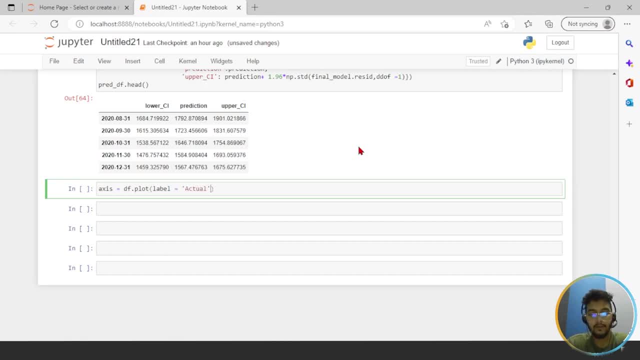 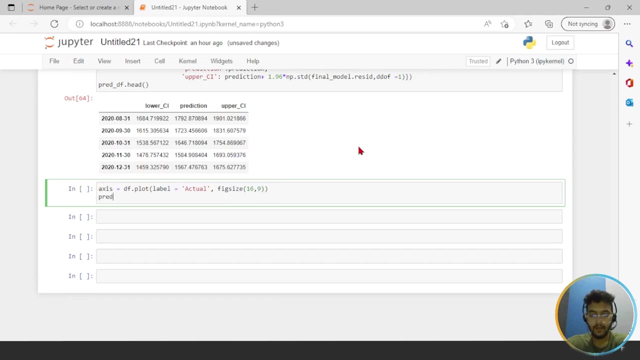 to actual comma figure size: 16 comma 9: prediction df dot plot. ax equals to this comma label. underscore df: it's lower ci. what i will do instead of this label. equal to forecast comma: alpha equals to 0.5. okay, this dot fill. this is lower. c is equal to 0.5. ok, that is what we will do instead of this label. equal to alpha equals to 0.5. okay, this dot fill. 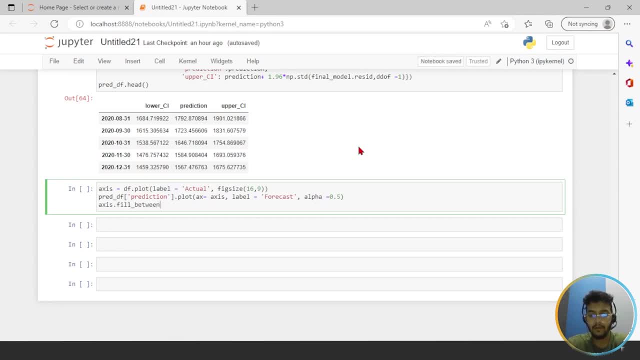 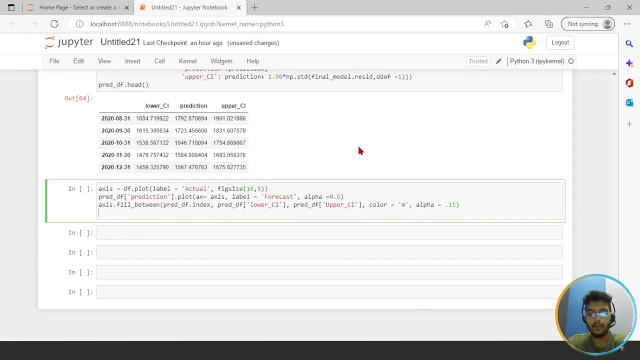 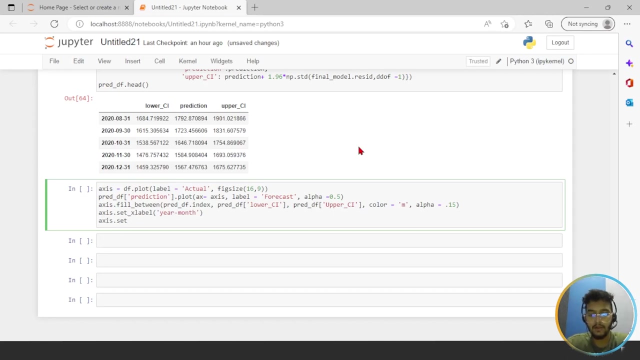 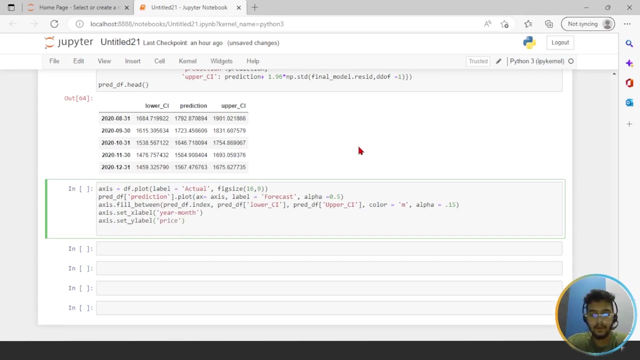 between: prediction underscore df: dot index: comma. prediction underscore df toward underscore ci: comma. prediction underscore df: this ci, then color equals to m, comma alpha equals to 0.15. okay then. axis dot set underscore x label: year, month. axis dot set y label: it's plt dot. 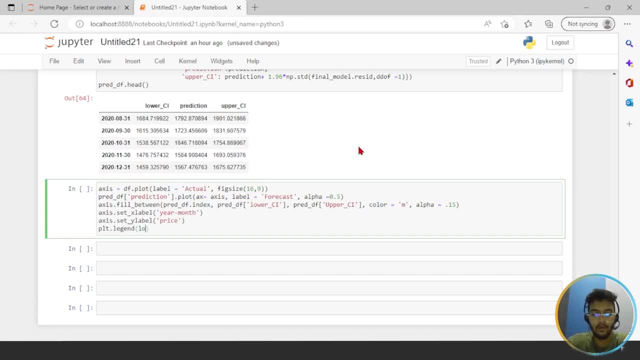 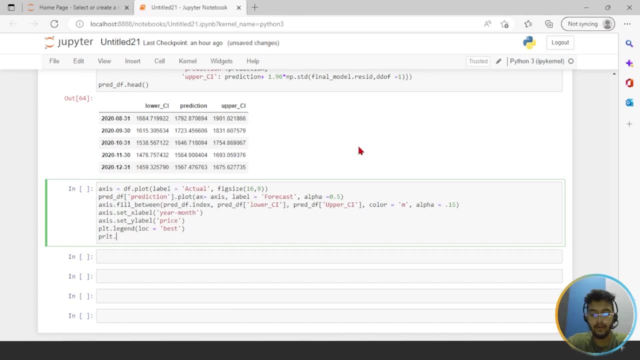 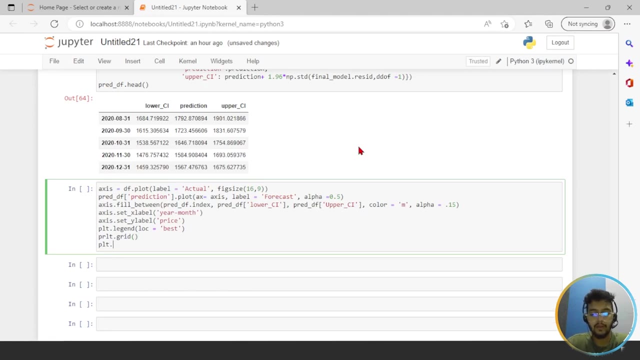 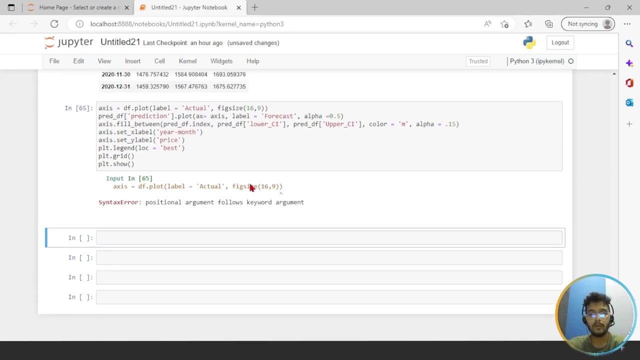 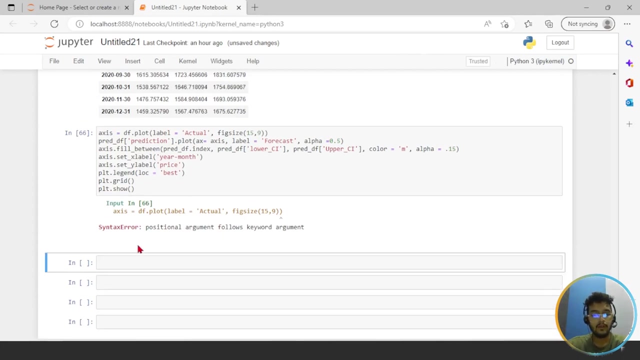 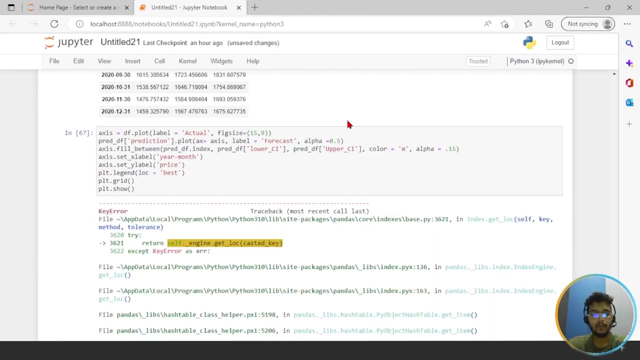 legend should be location question best then plt dot grid. plt dot show: okay, this is plt. only then press enter. okay, 16 comma 9 positional argument follows keyword argument 15: 15, oh, oh, okay, okay, i have to give you okay. okay, i have to give you. 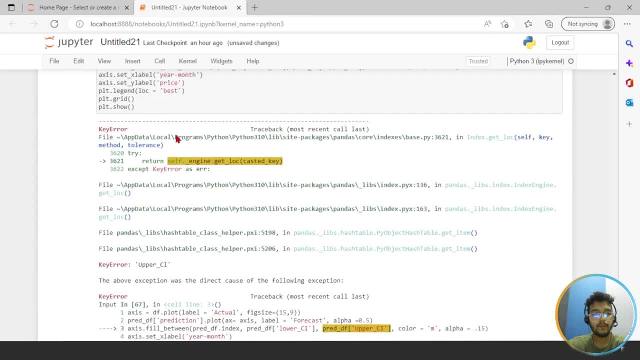 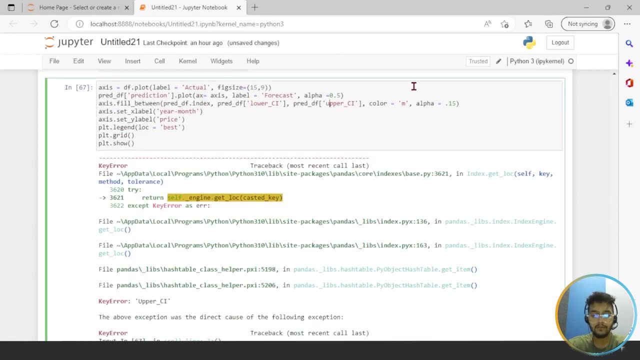 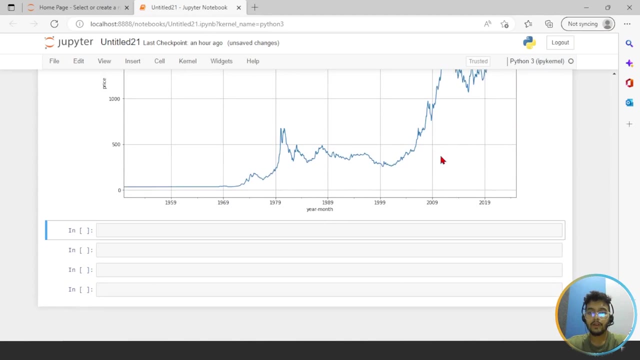 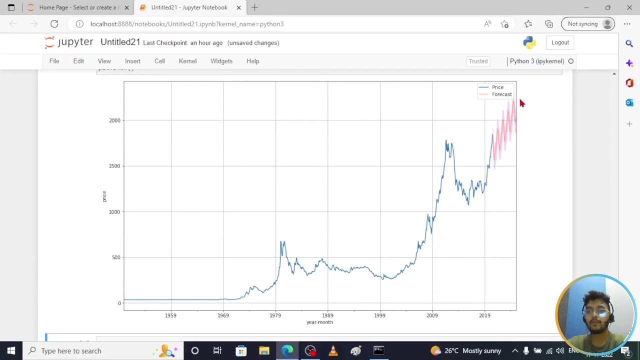 upper ci, upper ci, right, right. so here you can see our final model. so here you can see our final model forecasting. so till 2020 it is showing like normal, and after that, till till 20: 30. okay, this will be the forecast as per the data. 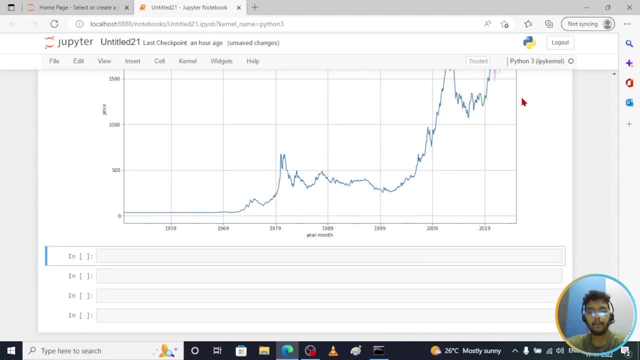 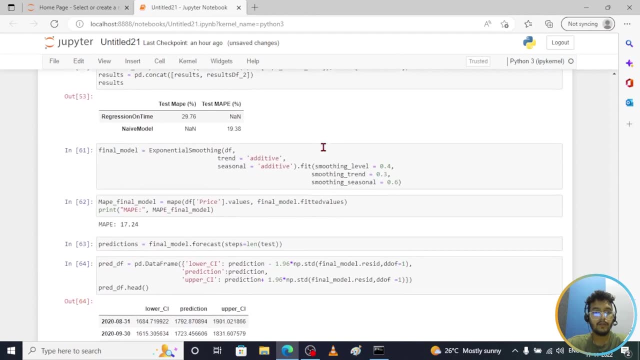 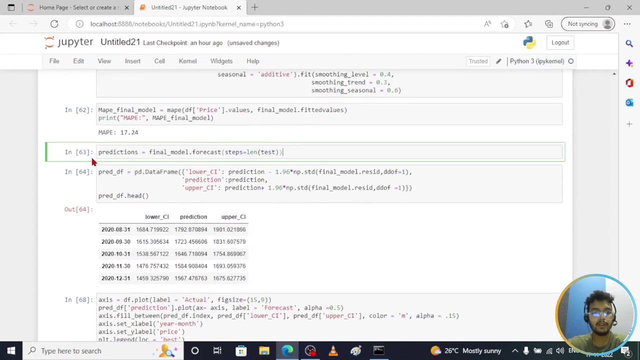 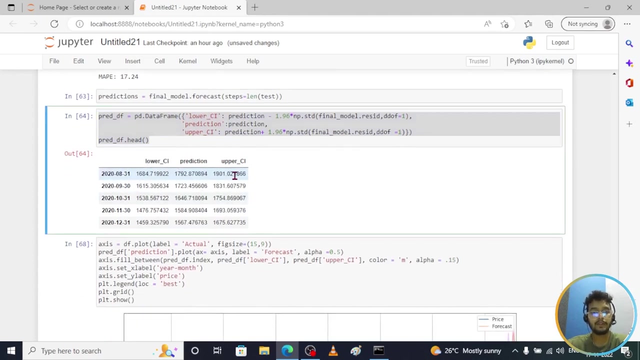 okay, so here you can see. you can see we have. the map is 17.24. okay then, here i did the prediction for the testing data and here i've created the data frames. these are the data frames: lower ci, prediction and upper ci, and then i have created: 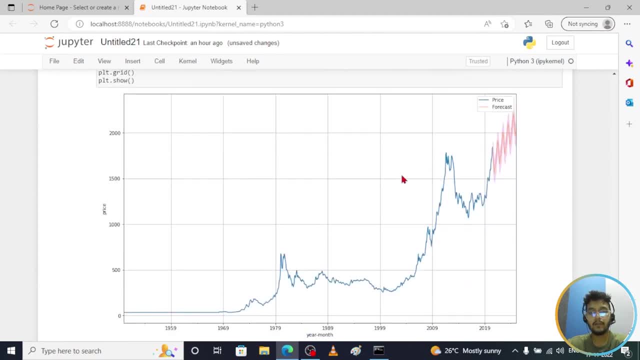 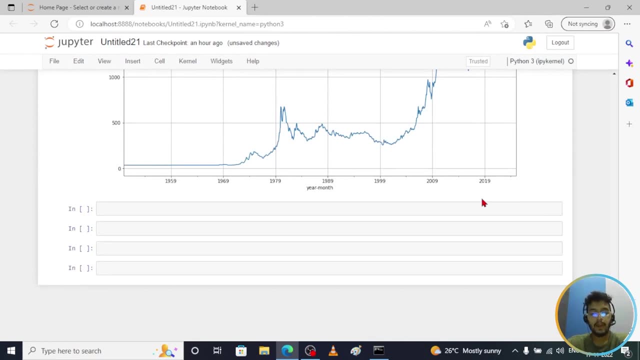 the and then i have created the final graph of the forecasting. okay, so i hope you guys must have understood, like, how you can do time series forecasting using machine learning or python, like. if you have any queries, you can ask in the comment section. our team will respond you as soon as. 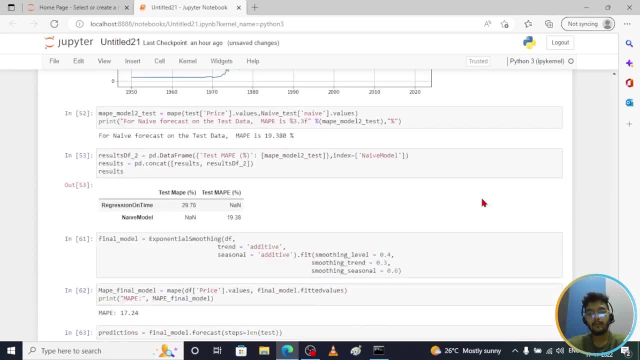 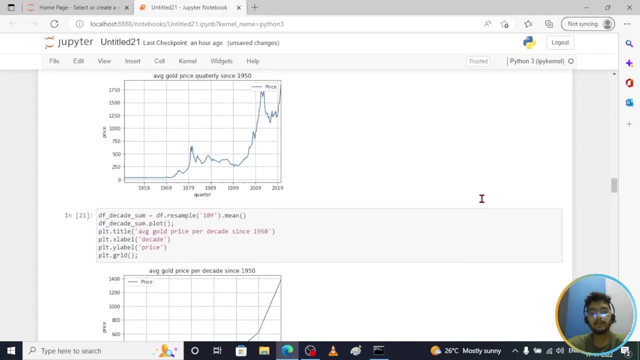 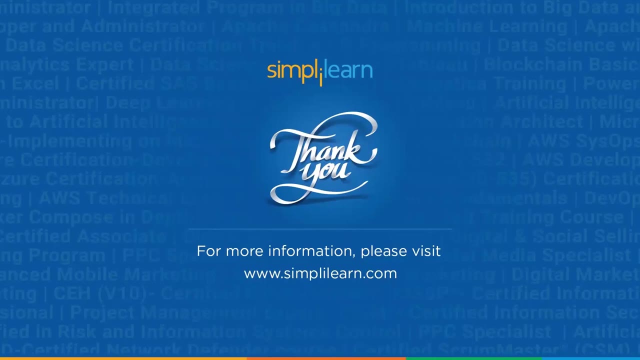 possible. or if you want this full code, this full code, just comment down for the same and you can download the data set from the description box below. and don't forget to check the course link from the description box below. and machine learning. thank you so much for being here. if you,